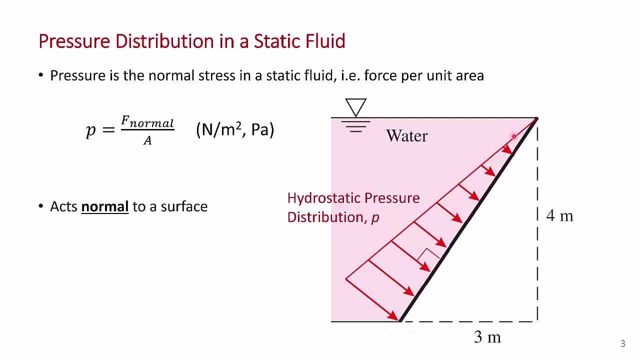 linear distribution later on in this video. So the pressure increases from zero at the surface and increases linearly. But the important point to notice here is that all of these vectors are perpendicular to the surface. So the pressure increases from zero to zero at the surface and 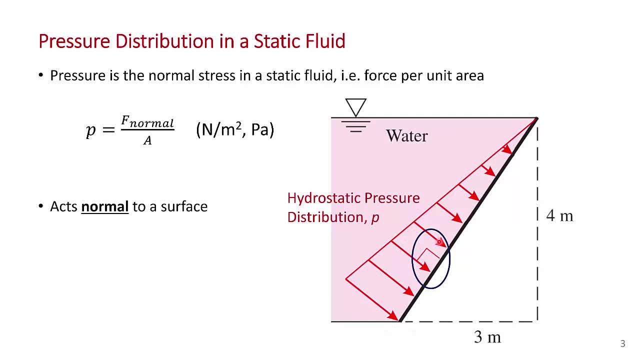 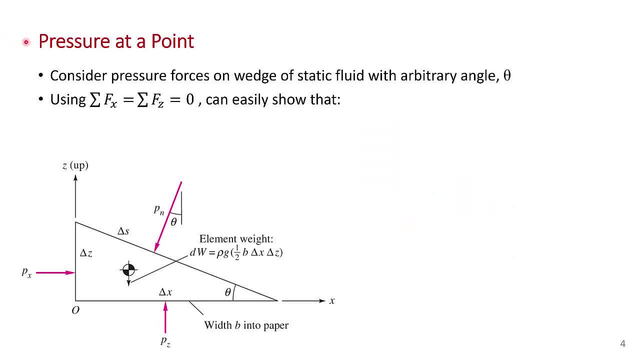 pressure force acts normal to the bounding surface. Now pressure is, it turns out, is independent of direction at a point. your book spends a lot of time talking about this. I'm just going to talk about it briefly because I think it's fairly straightforward. So if we consider an arbitrary wedge of fluid here, 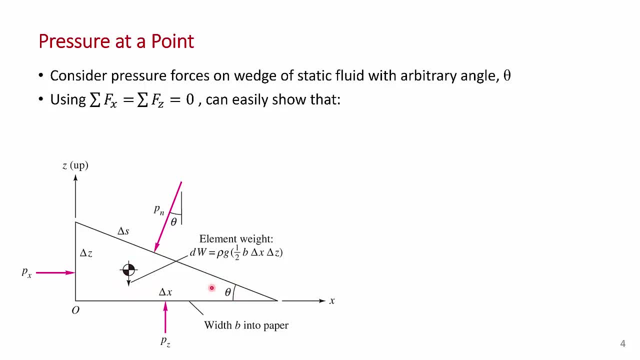 with an arbitrary wedge angle, theta, and we have a horizontal force- px, we have a vertical force- pz, And on this inclined face, which is at an arbitrary angle- theta, we have some force. we already talked about the pressure force acting normal to that surface. So we have 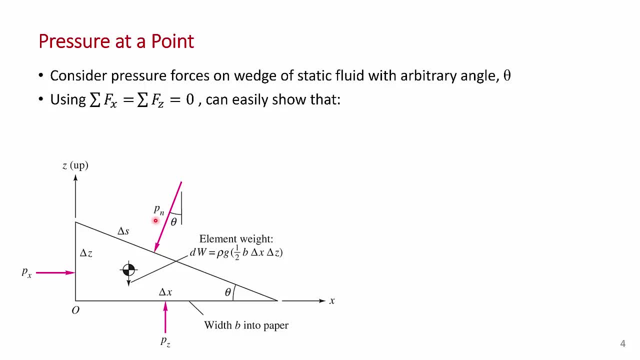 some force pn. If you do a simple static equilibrium on that wedge- and you can look it up in your book- if you do, the some of the forces in the x and some of the forces in the vertical direction are zero. you can easily show that you come to the result that 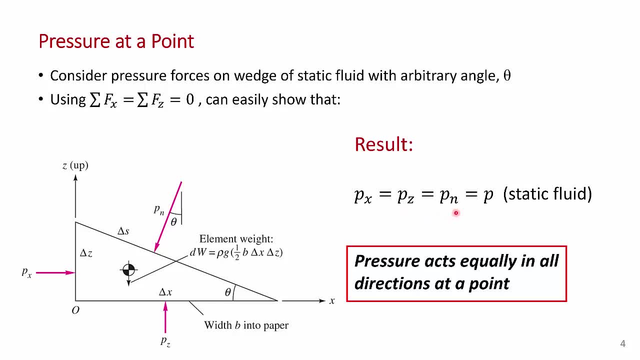 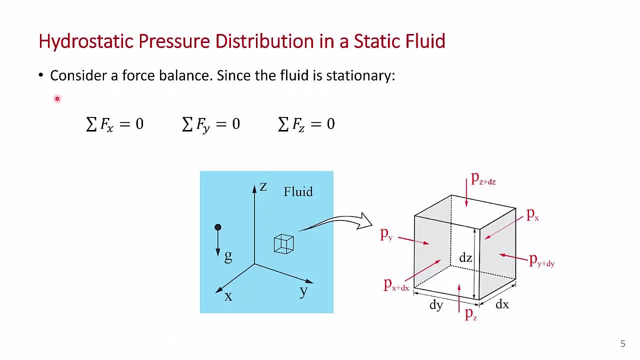 px equals pz equals pn, which is the force at any arbitrary angle, equals just p. So the point of this is that pressure acts equally in all directions. So next I'm going to do a little bit calculus to determine the differential equation for the hydrostatic pressure distribution in a static. 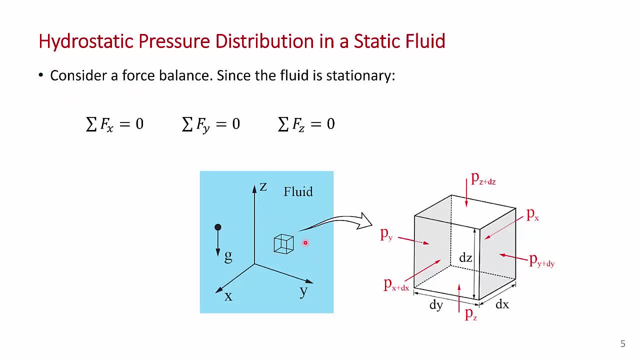 fluid. And we're going to do that by considering a little elemental volume of fluid with dimensions dx, dy, dz, and look at the pressure forces on it and set the sum of the forces in the x, y and z direction zero, because of course this is a static fluid. 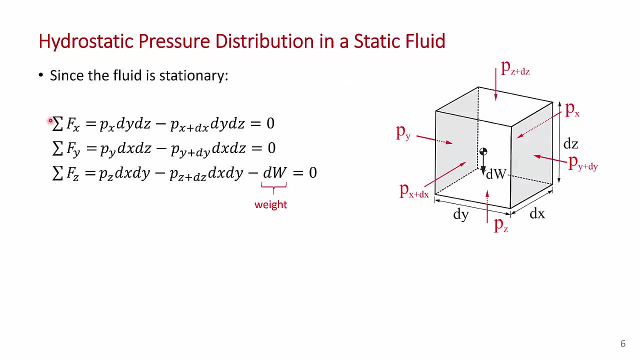 So, since the fluid is stationary, we can set the sum of the forces in the x, y and z directions to zero. And what we have here is on this back face. here we have a force- px- acting in the x direction and then a little bit moving in the x direction a distance- dx. we have a force acting in the negative. 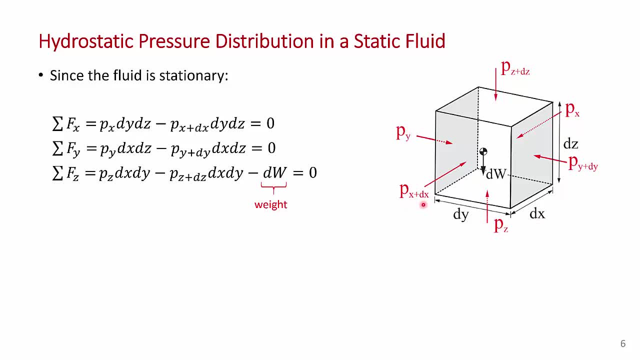 x direction p at x plus dx, And similarly we have forces in the y, y plus dy, z, z plus dz. So if we apply static equilibrium to this fluid element, we get these following equations here: x and y are pretty straightforward. Notice the area. so. so pressure times. area is force, So 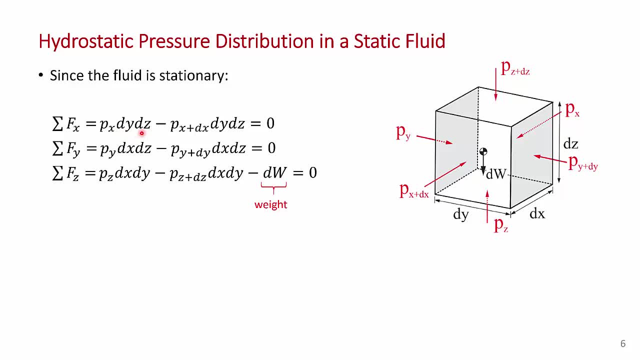 px times dy, times dz. That's the area of the back face here dy times dz. Similarly, the front has the same area. So we can apply that in the x, y and z directions. The difference of course in the dead direction is we have we have the weight of the element, So the difference in the pressure 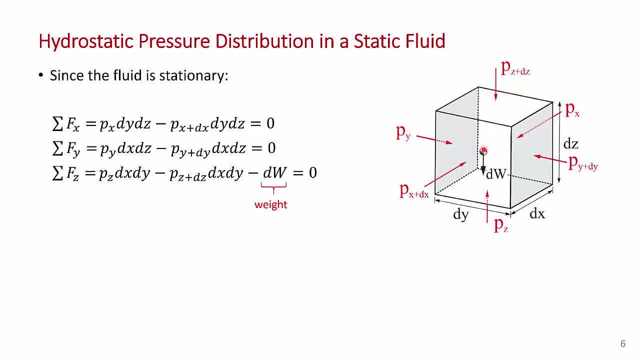 forces on the top and bottom faces has to pass the balance, the weight force. And that weight force is just g, y and z times the differential mass. so gdm and dm is density times volumes, or density times differential volume, and the differential volume is dx, dy, dz, So that's the differential weight. 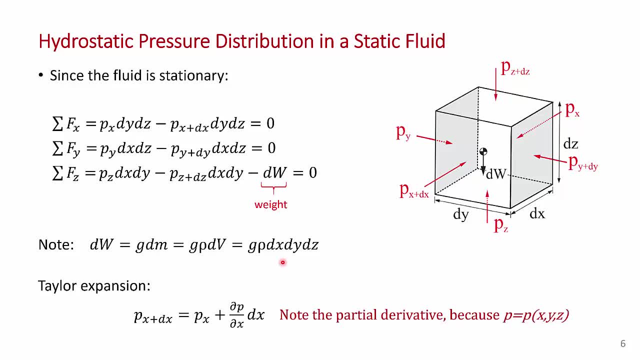 term. Now, what I'm also going to do when I do this derivation is for these terms on the faces at x plus dx, y plus dy and z plus dz. I'm going to make the substitution using a simple Taylor expansion, So p at x plus dx equals p at x plus dy, p by dx times dx, And I'm going to make: 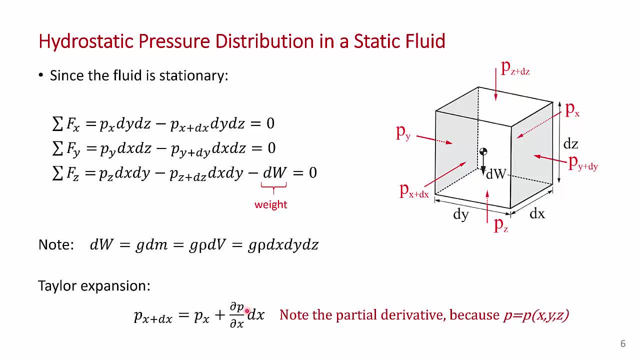 that substitution into the x equation. Before I move on, I should point out that I'm using partial derivatives here. Notice these are not full derivatives, they're partial derivatives. that's because pressure is a function of the three spatial coordinates x, y and z, So making 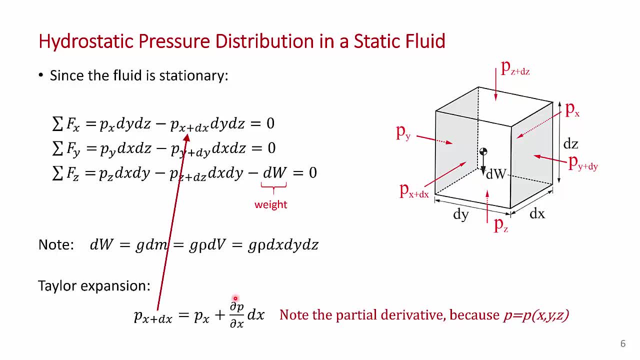 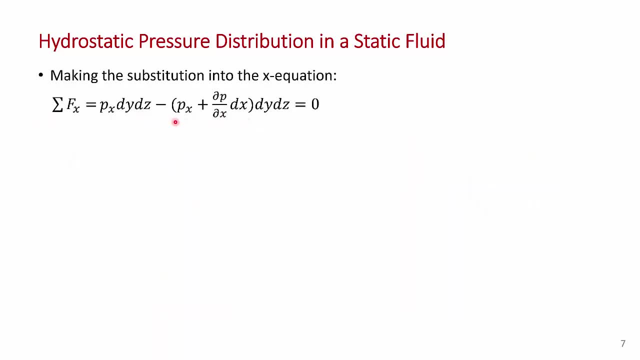 that substitution, move to the next slide and just look at the x equation. So that's what I've done. This is the x equation And I've made the substitution here for p at x plus dx using that Taylor series expansion. Now we can rearrange this, we can move this term over to the right. 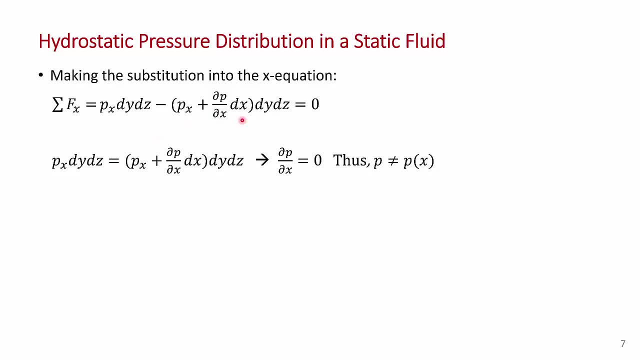 hand side. That's what I've done here. I've just moved this term over to the right hand side. After making that arrangement, we can see that p at x dy dz on the left hand side and we have p of x dy dz on the right hand side. So that cancels. 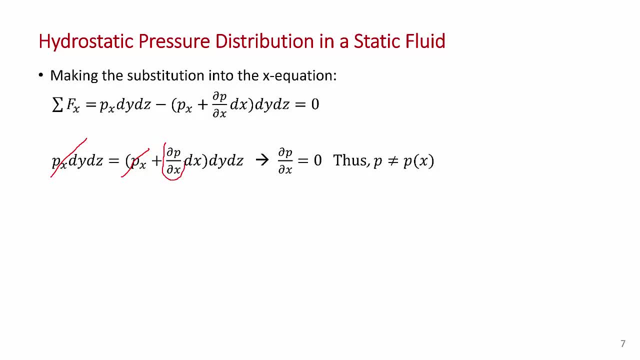 with that And you can see that you end up with just this term. So you end up with dp. dx is zero And that tells us that the pressure is not changing in the x direction. So p is not a function of x. Now, if you go back and look at the equations, you can see. 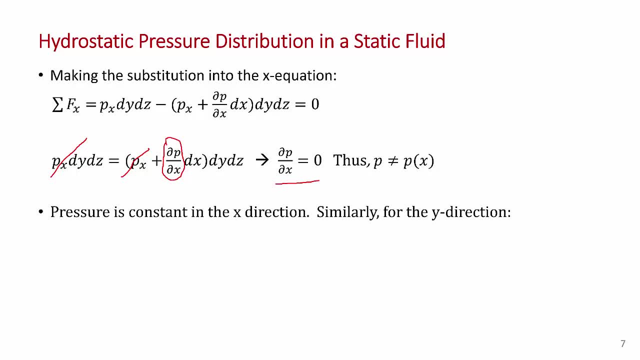 you can do exactly the same thing in the y direction. You can come up with the same result: that the pressure doesn't change in the y direction. So dy p, dy y is zero. Next we'll consider making that substitution in the z direction. I've made the substitution here for the. 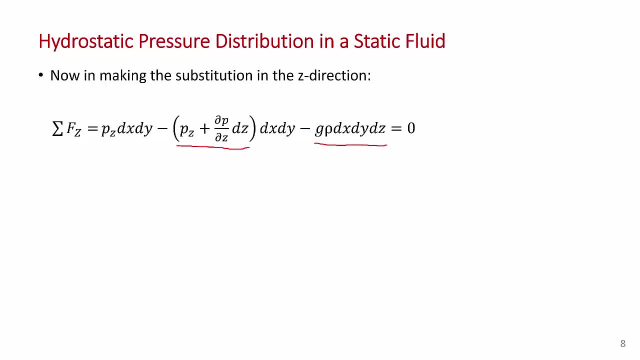 Taylor series expansion. And here's the differential weight term. You can see that this term p z dx dy cancels with this term P z dx dy And if you simplify this you just get that die p by day z equals minus rho g And now we can switch to full derivatives because we've shown that pressure. 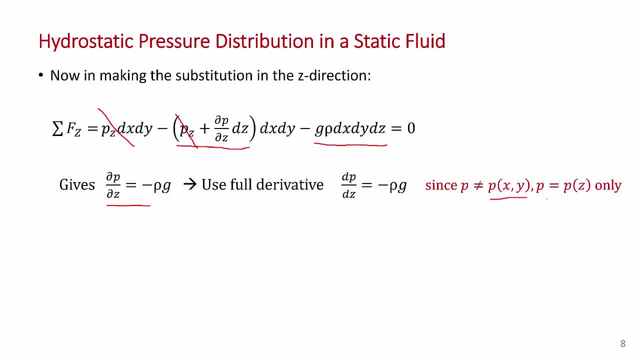 is not a function of x and y, it's only a function of a single variable. So we can change to these change to a full derivative and we end up with our differential equation for the pressure distribution. as static fluid is, is di P, die z equals minus rho g. Now if we assume that rho is, 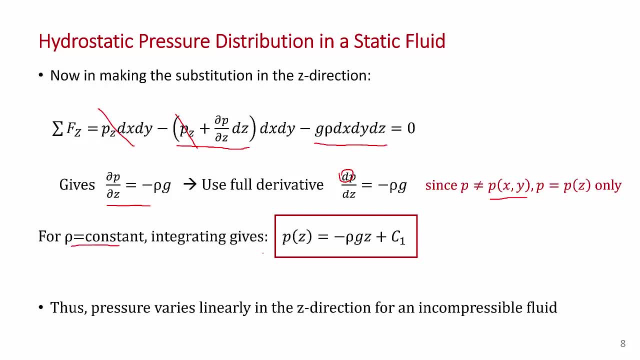 a constant. so if we assume a liquid, we can integrate this very simply and just separate the variables and you get that the pressure is minus rho, g, z plus some constant and z is the vertical coordinate. So this negative sign here indicates that pressure decreases as you go up. 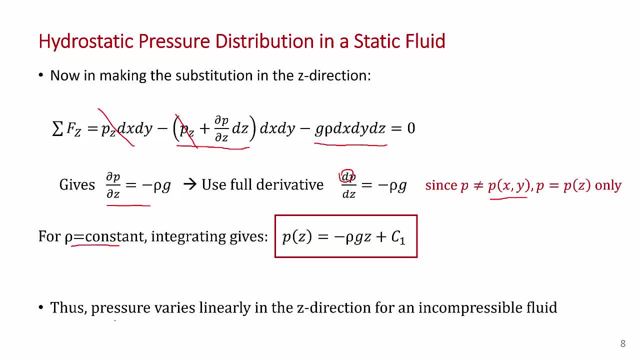 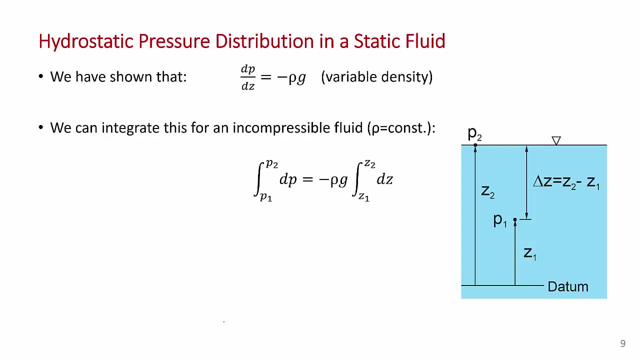 And so not only does pressure decrease when we go up, but pressure decreases linearly in the z direction for an incompressible fluid. So we just showed that di P, die z equals minus rho g, and that applies for constant as well as variable density. One thing we can do is integrate that expression for 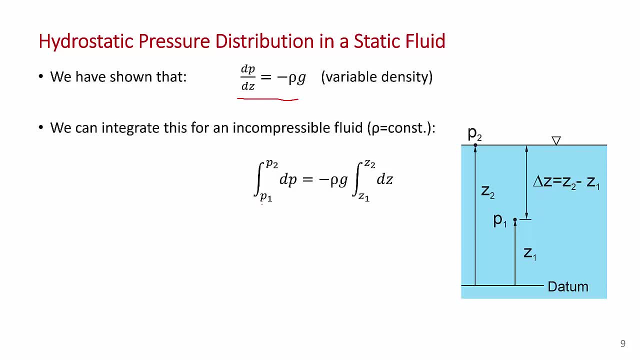 an incompressible fluid And it's a little easier if we integrate it as a definite integral. So we integrate, So we consider some fluid here- here's the free surface up here- And we consider point one at elevation z one and point two here at elevation z two And we can evaluate the. 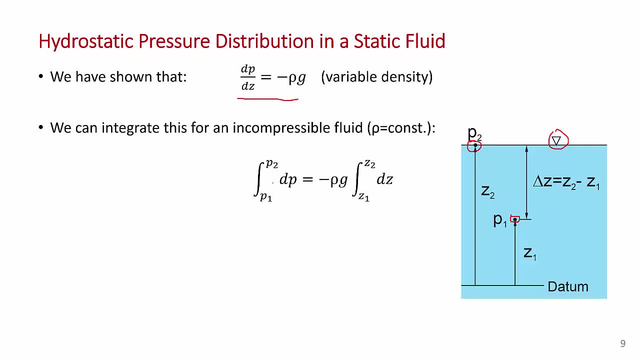 pressure difference p one minus p two. So we integrating here. what I've done is separated the variables and I'm integrating from p one to p two and from z one to z two. it's a very straightforward integration If we assume 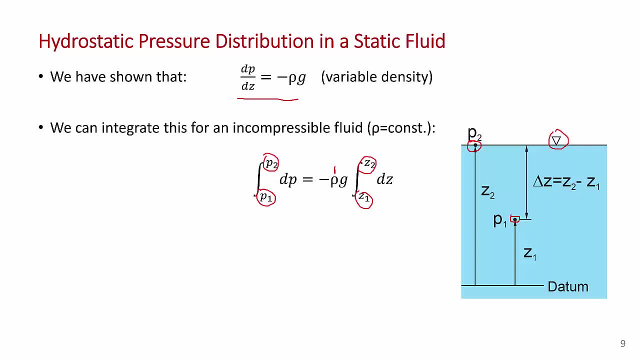 that density is a constant. we can bring the density here outside of the integral and the integration becomes very straightforward. So we just get p two minus p one equals minus rho, g, z two minus z one And making a little bit of rearrangement we can solve for for p one here. 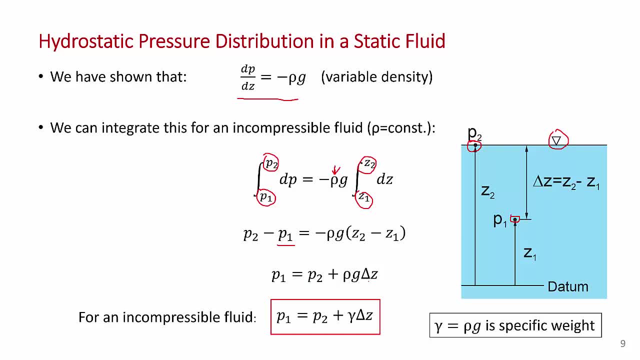 we get that p one equals p two plus rho g, delta z. Now rho g, we learned in chapter one, is a property on its own called specific weight, And so the pressure at one, pressure at some depth, is just the pressure of the surface: p two plus gamma times the depth of the point of p one. 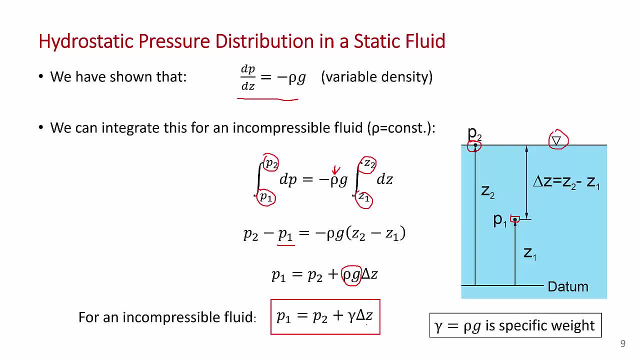 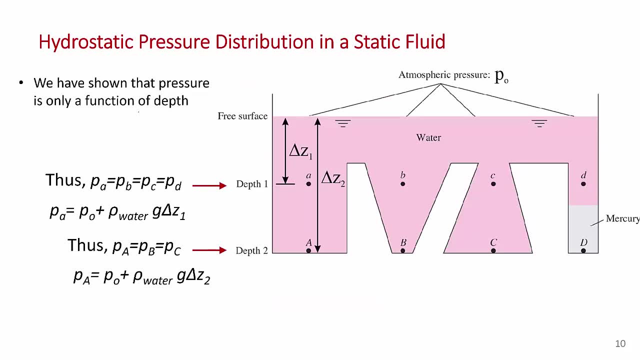 So pressure increases as we go down in the fluid. So in the previous slide we showed that pressure is only a function of depth. delta z. So if you consider a reservoir here with a funny shaped bottom, here you can consider points A, B, C and D. they're all at the same depth in the same fluid. delta z one. 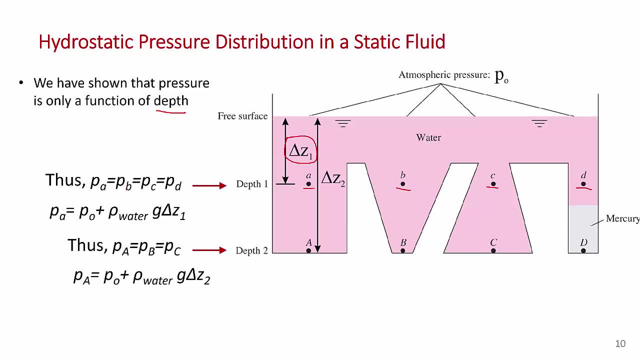 know from our previous analysis that the pressure at A, B, C and D are the same And that's equal to the pressure of the free surface, p not- which would normally be atmospheric pressure, plus the gamma of water. So rho water times, g times that depth, So the pressure that the at these 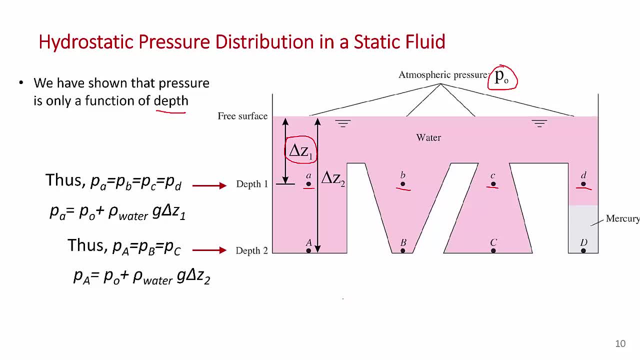 four points are all the same. Similarly we consider that. consider the capital letters here at point capital A, capital B and capital C. they're also at exactly the same pressure because they're at the same depth in the same fluid water. delta z two, that's equal to. 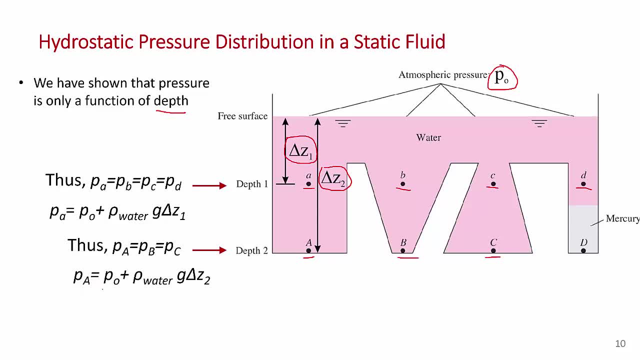 so PA equals PB equals BC, which is the free surface pressure plus the gamma of water, times that depth. Now you might have wondered why I didn't include point D over here. So the question is: I just talked about pressure being a function of depth alone. Does the 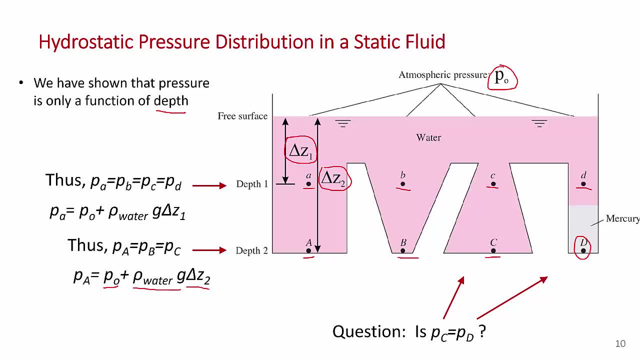 pressure at C equal the pressure D? I want to pause the video and just think about it for a moment. The answer is no, And the reason is is because point D over here is in mercury, and mercury has a high temperature. It has a higher density than water, substantially higher density, And so the pressure D is going. 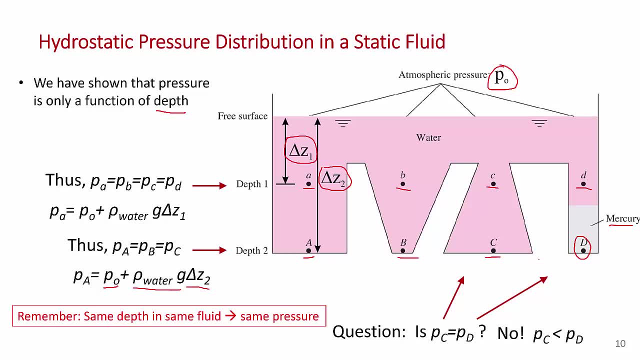 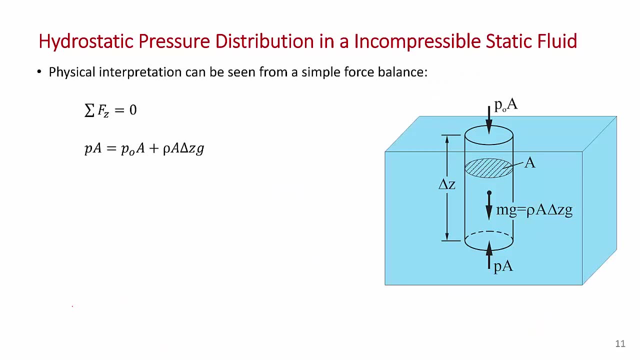 to be higher than at C. we're going to do some calculations of that type in this chapter, So remember that if you're in the same depth in the same fluid, you have the same pressure. Now I just finished doing some calculus And but I just want to do a non calculus interpretation. 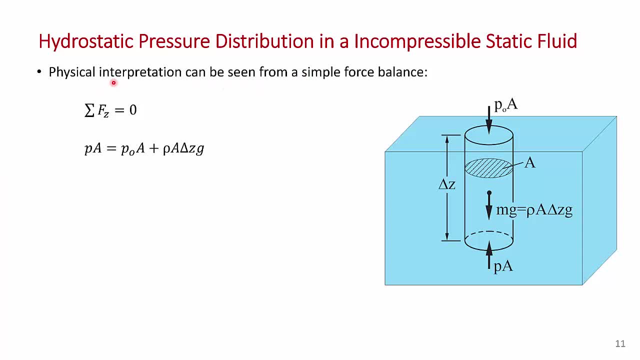 here. So this is a simple interpretation, Just using a force balance. So consider a body of, let's say, water here, And I'm considering a column of water, a cylindrical column of water that goes all the way to the surface. You can do a simple force balance on that that. the pressure at the bottom times, the 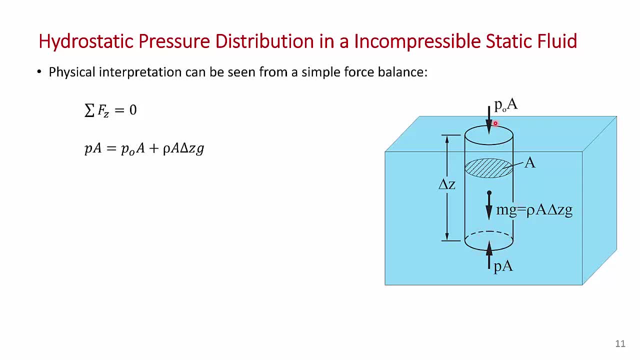 area, the cross sectional area, which is arbitrary, and the pressure at the top here, the atmospheric pressure times area. the difference in those two pressures must balance the weight And the weight of this column, if the area of this column, if the area of this column is. 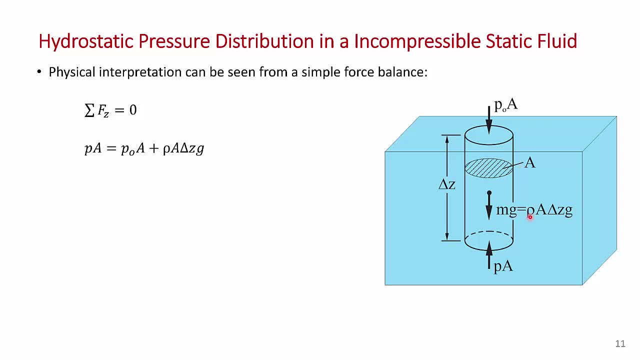 cylinder is a, then it's going to be rho a. delta z is the height times g, that's the, that's the weight of this column of water. And you can do a simple force balance, that that PA at some depth. at some depth, delta z PA has to balance the pressure force on. 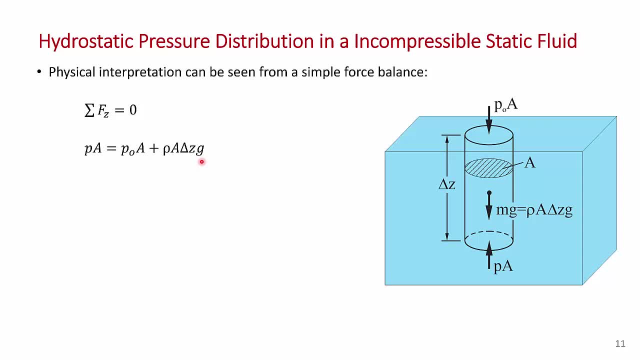 the top plus the weight of the of the column of water, And if you solve for for the P, you just get it's P naught, P two minus P naught plus rho g, delta z, which is exactly the same result we had before when. 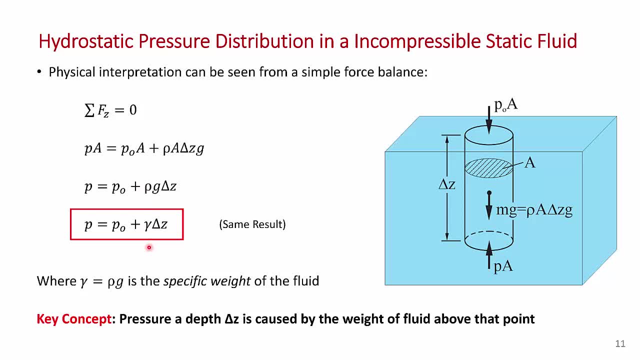 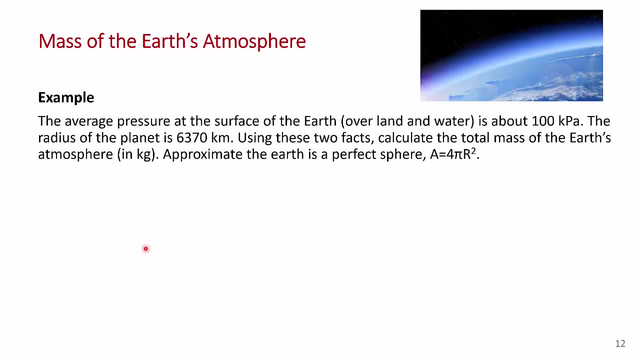 you make the substitution that rho g equals gamma, which is the specific weight of the fluid. So the key concept here is the pressure at a depth. delta z is caused by the weight of fluid. above that point And using that concept we can do some interesting calculations. For example, it's surprisingly: 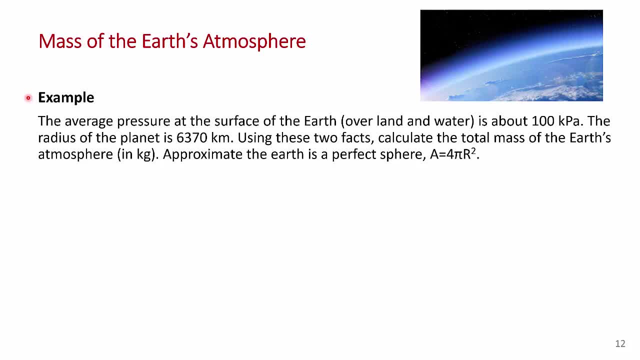 easy to calculate the weight of the fluid above that point. I think it's quite easy calculate the mass of the Earth's atmosphere And the question states: the average pressure at the surface of the Earth over land and water is about 100 kPa. The radius of the planet is 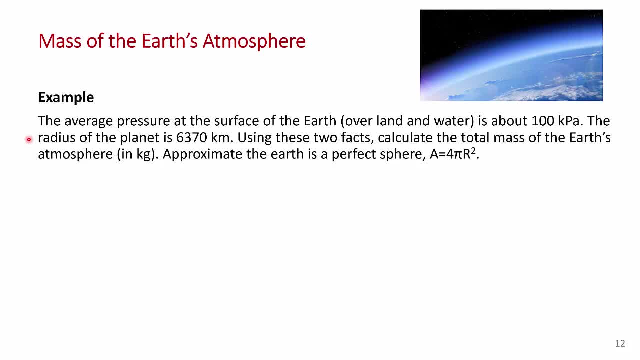 6,370 kilometers. Using these two facts calculate the total mass of the Earth's atmosphere. So all the air in the Earth's atmosphere approximating the Earth as a sphere. It's very close to a sphere. It's a slightly oblate spheroid, but that's a pretty good. 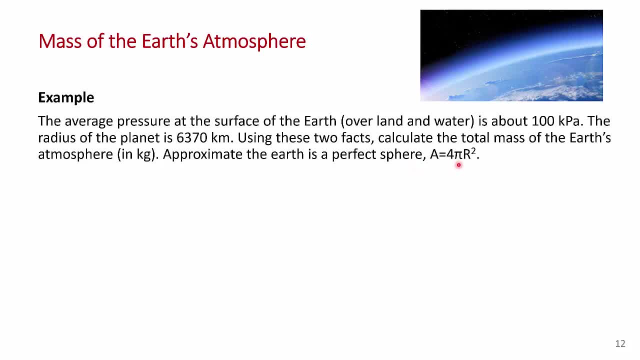 approximation, So we can use the area as 4 pi r squared. So the solution here is based on the concept that we just discussed that the atmospheric pressure is caused by the weight of the air. So it's the weight of the air that produces the pressure at the surface. And if we do a free body, 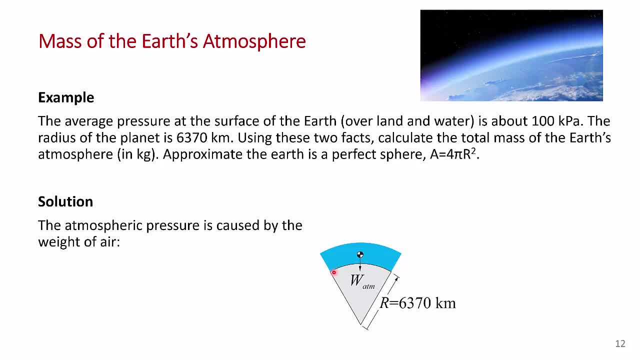 diagram. of course, here I'm just considering a portion of this sphere. I'm going to apply over the entire sphere, of course. So the weight of the atmosphere is balanced by the atmospheric pressure times, the surface area, That would be the surface area of the planet From this free. 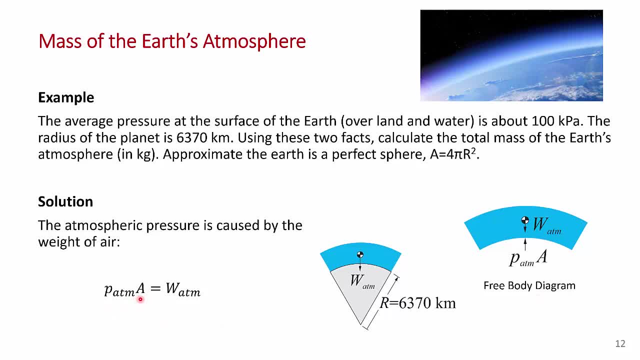 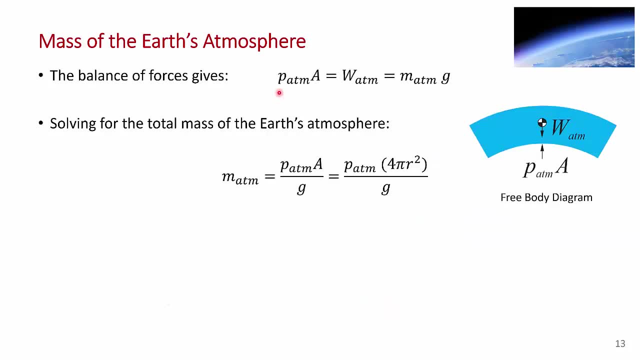 body diagram, we get that p atmosphere times the area of the planet equals the weight of the atmosphere. Okay, and so we have that the weight of the atmosphere is balanced by the pressure force. p atmosphere times the area of the planet, Of course the weight of the atmosphere is. 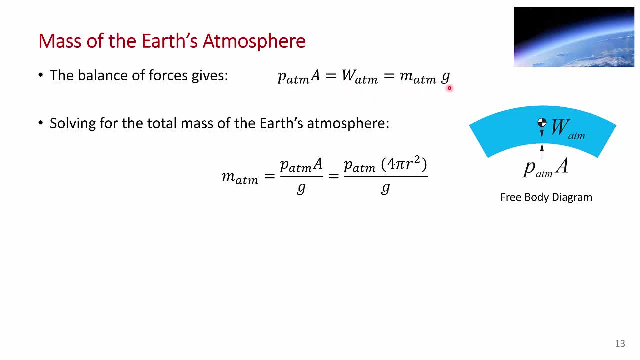 the mass of the atmosphere, which is what we're after times g, And so we can solve for the mass of the atmosphere the atmospheric pressure times the surface area of the planet We're going to approximate as 4 pi r squared divided by g, So now we can make the substitutions Atmospheric. 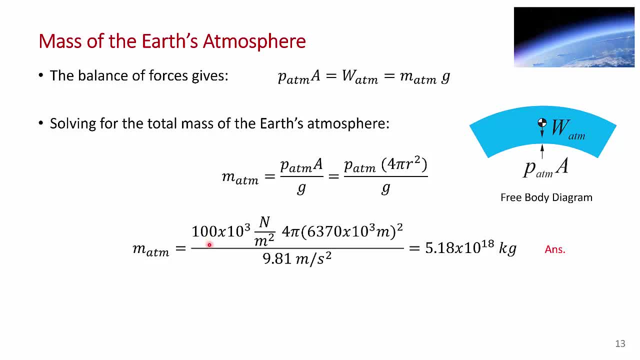 pressure, averaging at 100 times 10 to the third pascals, 4 pi, and there's the radius of the planet, 6,370 kilometers. So that's 5 pi r squared divided by g, and you end up with 5.18 times 10 to the 18 kilograms, a huge. 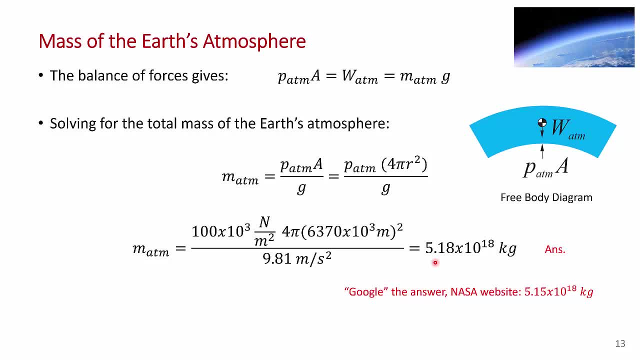 number. I tried googling that answer and the NASA website gives 5.15 times 10 to the 18 kilograms. So that's pretty amazing that with such a simple calculation we can get the total mass of air in the atmosphere to within about 1%. So the key concept here and the reason I did this example: 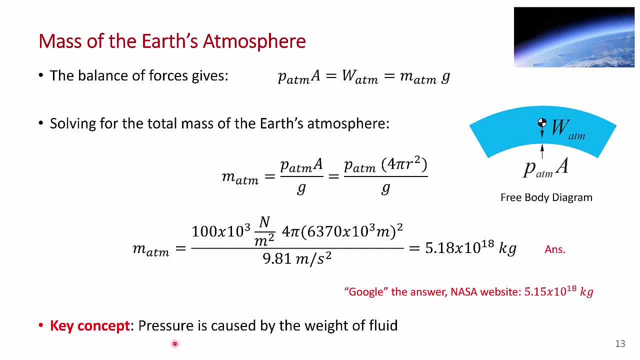 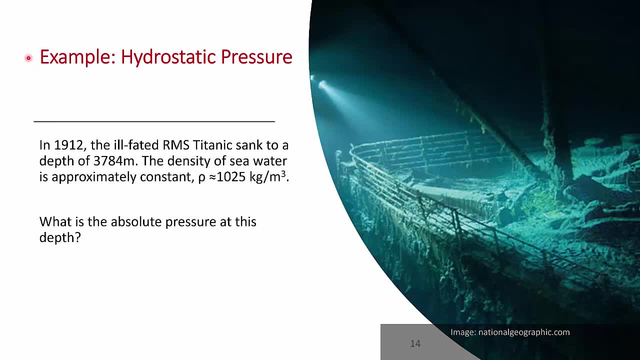 is to emphasize that pressure is caused by the weight of the fluid above. So I just want to do another simple example just to solidify the concepts. So of course, the Titanic sank off the east coast of Canada, just a little bit south of Newfoundland, in 1912. And it sank to an 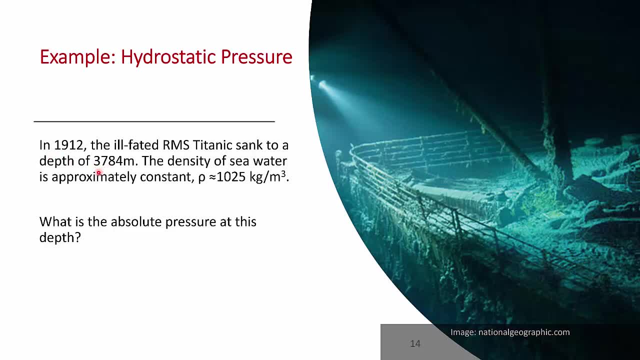 enormous depth, almost 3.8 kilometers here, 3,784 meters, And we can take the density of water to be sea water to be 1,025 kilograms. That's a little more dense than freshwater because of the salt content. 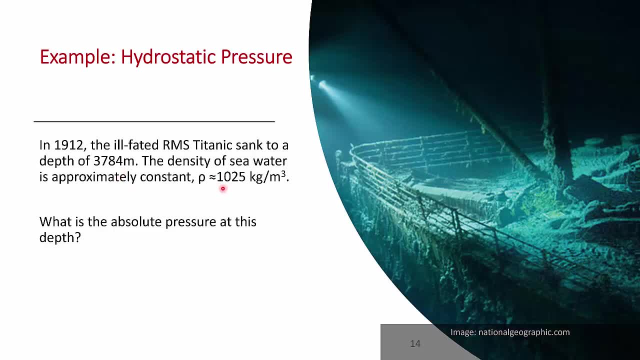 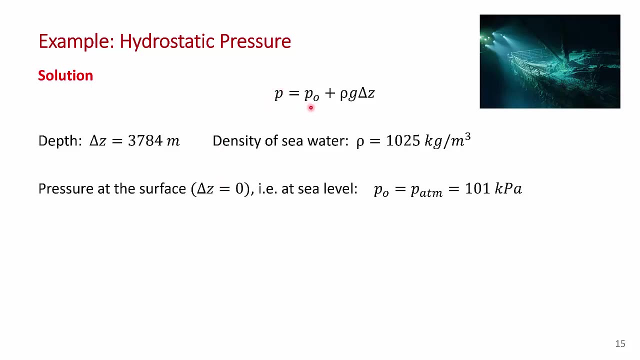 So, using those two numbers- the depth and the density of seawater- let's calculate the absolute pressure at the deck of the Titanic. So it's a fairly straightforward calculation. The pressure at the deck of the Titanic is equal to the atmospheric pressure at the free surface. 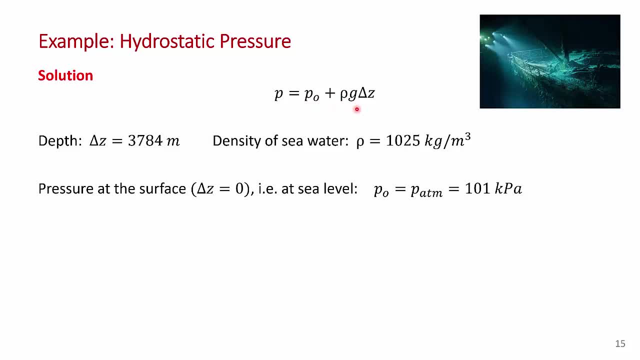 at the surface of the water and then gamma of water times the depth. We were told in the problem that the Titanic is at 3,784 meters and the density of seawater is slightly greater than freshwater, And we're going to take the pressure at the surface to be 101 kPa. So it's simply 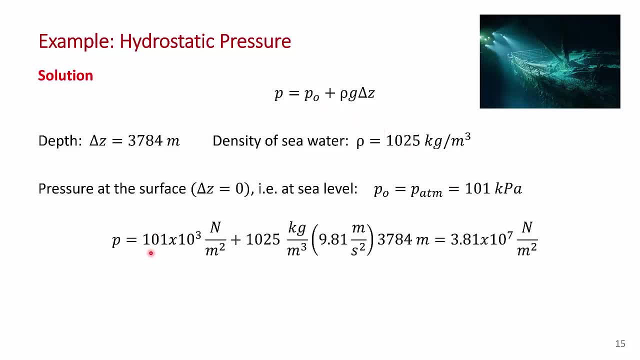 making the substitution. So there's 101 kilopascals Density of water g and the depth delta z. And you can see here, check your units, that kilogram meter per second squared is a newton and that meter is going to make that. 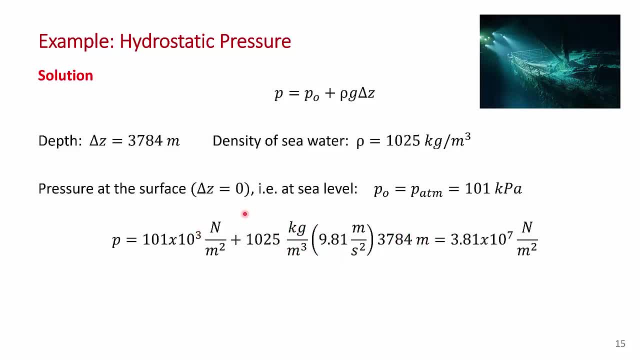 meter squared, So we've got newtons per meter squared, so we can add these two together. I really recommend you always check your unit's balance. When you do this calculation you get 3.81 times 10 to the 7 pascals, So that's 38.1.. 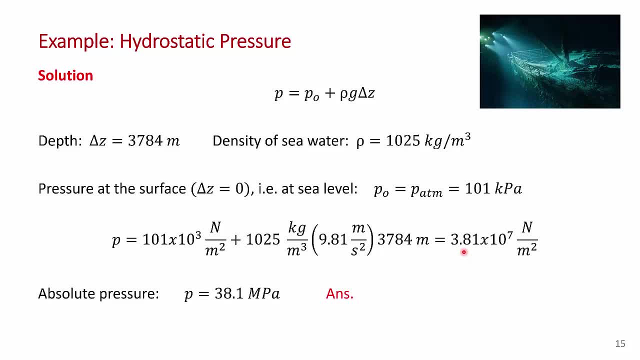 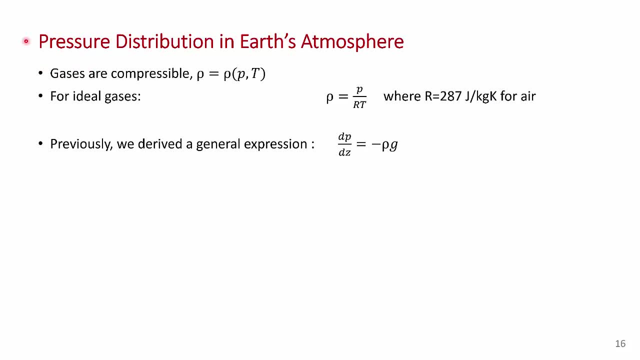 So that's 38.1 megapascals, which is about 380 atmospheres. It's quite an amazingly high pressure. So next I'm going to talk about the pressure distribution in fluids that are compressible, so in other words in gases, And specifically I'm going to talk about the pressure distribution. 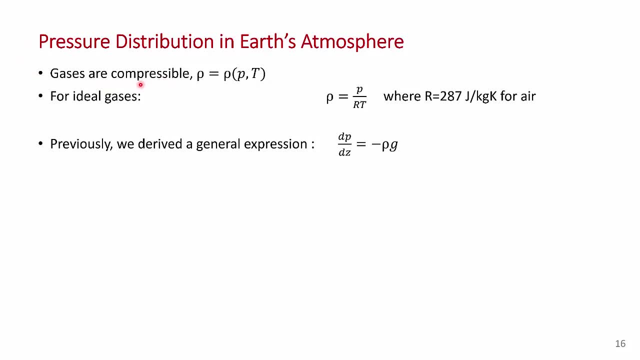 in the Earth's atmosphere. So the difficulty with finding the pressure distribution in gases is that the density is not constant. It depends on the temperature. It depends on the temperature. So the temperature changes as you go up and down the equation. So if 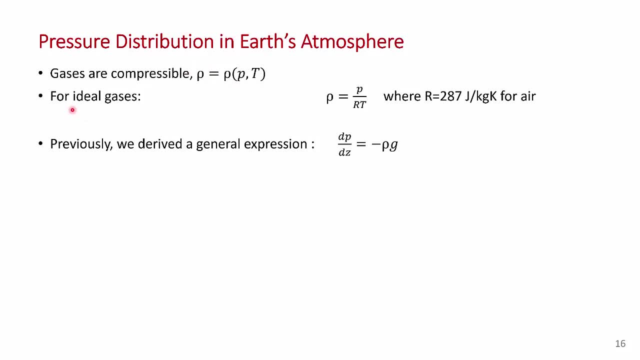 it depends upon the pressure and temperature. Of course, for air in the atmosphere we can approximate the density using the ideal gas equation of state. So rho equals p over RT, where the gas constant for air is 287 joules per kilogram k. Previously we showed that 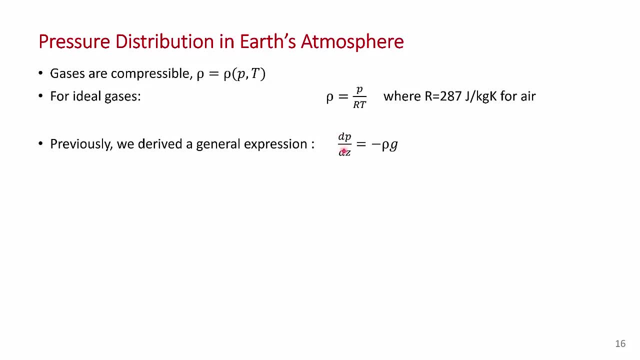 we did a little bit of calculus to show that the rate of change of pressure with altitude is equal to minus rho g. So pressure decreases as we move upwards, And so now to integrate this, we have to include variable density here. So what we're going to do, 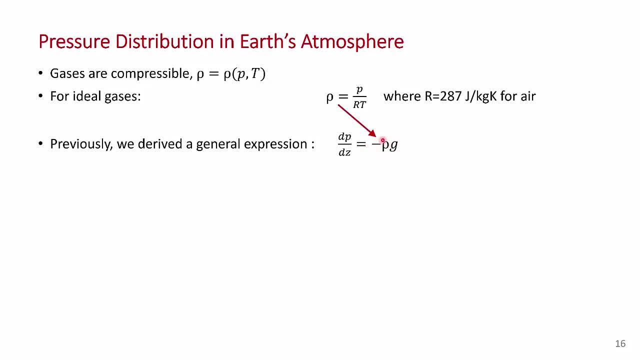 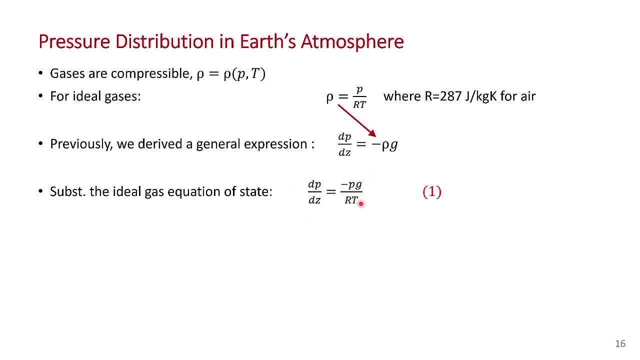 have to do that. The difficulty in integrating this is we have to make some assumption with respect to temperature. Now, in the troposphere the temperature decreases with altitude And it's a pretty good approximation that it decreases linearly. It's called the. 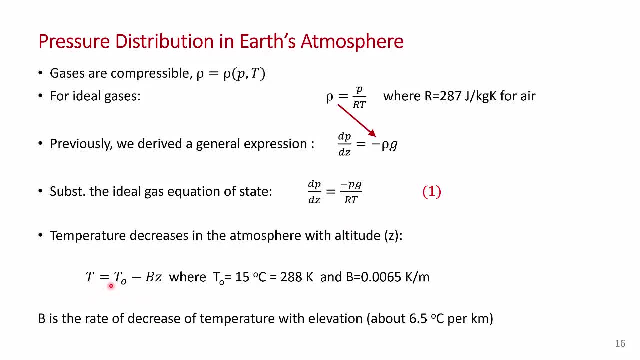 adiabatic lapse rate. So the temperature is equal to the temperature of the surface, minus some constant times z. So it is constant slope And to a very good approximation. the adiabatic lapse rate is equal to the temperature of the surface, minus some constant times z. 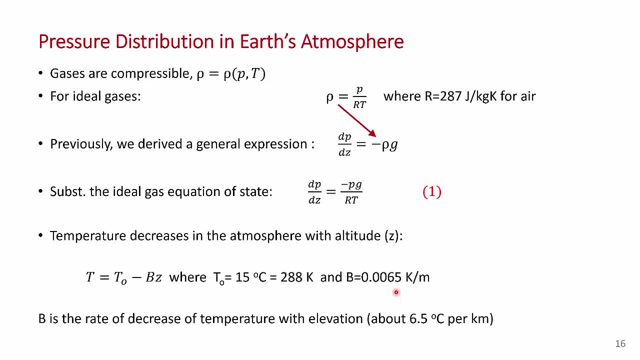 The adiabatic lapse rate is about six and a half degrees per kilometer. So for every kilometer you go up, the temperature decreases by about six and a half degrees, And so we're going to make the substitution in here for the temperature. This is very close approximation in the 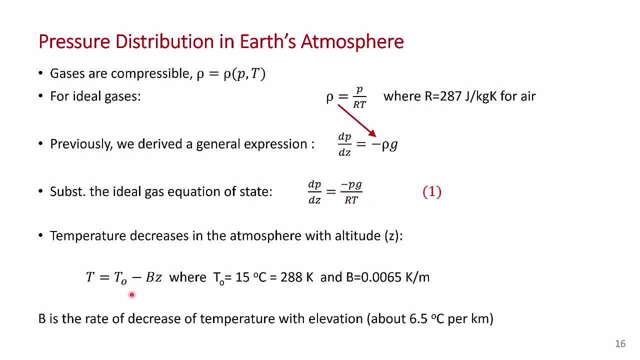 troposphere. So in the first 11 kilometers the temperature varies linearly with altitude. Of course it varies locally based on local weather conditions, But on average around the globe temperature decreases linearly with altitude at about six and a half degrees per kilometer. 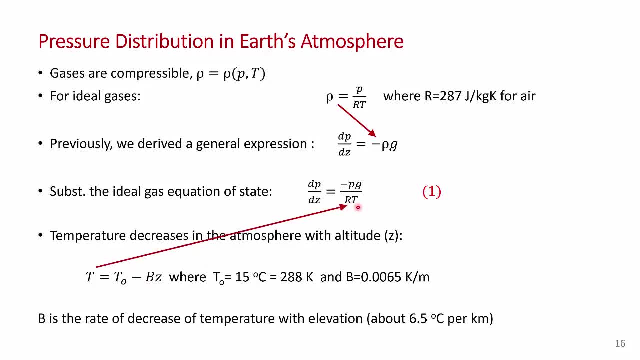 So we're going to make the substitution for t in here, and then we'll be able to perform our integration. So that's what I've done. on the next slide, I've just made the substitution to equation one for this linear variation, Oh, and I've also separated the variables. So pretty straightforward. 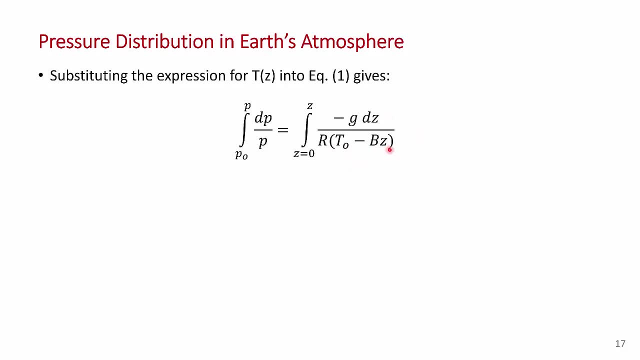 I've just separated the variables And there's your adiabatic lapse rate, And I'm doing this as a definite integral, And then I'm going to make the substitution for t in here, And then I'm going to make the substitution for t in here, And then I'm going to make the substitution for t in here. So 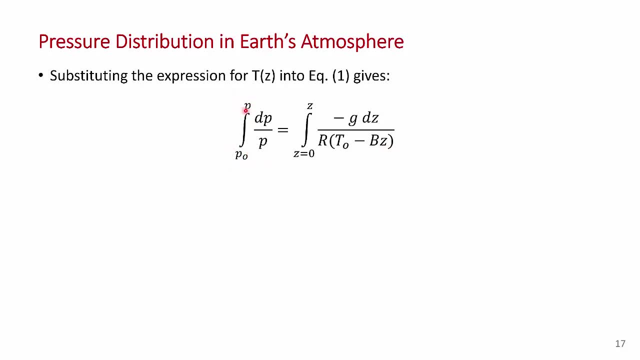 I'm integrating from the surface to some arbitrary altitude where the, where the pressure is b. So I'm integrating from ground level, which is z equals zero, to some arbitrary altitude, z. Now this is not totally straightforward, but not terribly difficult. integral, If you're comfortable. 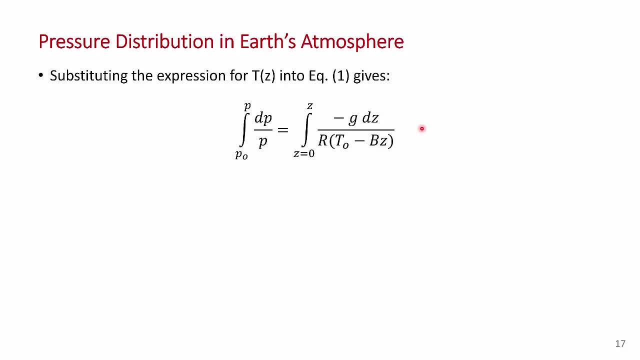 with your first and second year calculus. I won't go through the details, It's not that important to the course. If you do this integration, you get that the pressure varies as p naught. and then you get this term here where g upon R, b is a constant gravitational constant, b is your adiabatic lapse. 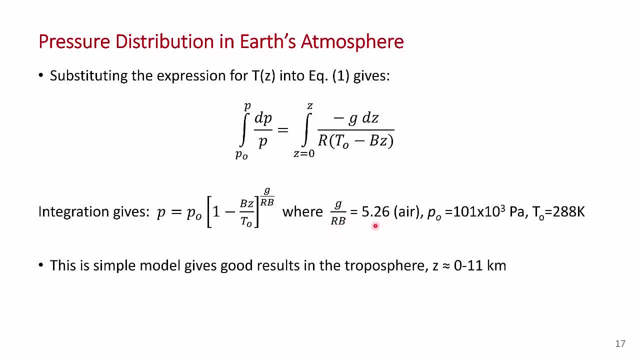 rate and R is the gas constant. for air, it turns out to be 5.6. for our atmosphere, p naught is the surface pressure, which is we're going to take as 101 kilopascals And by standard agreement. 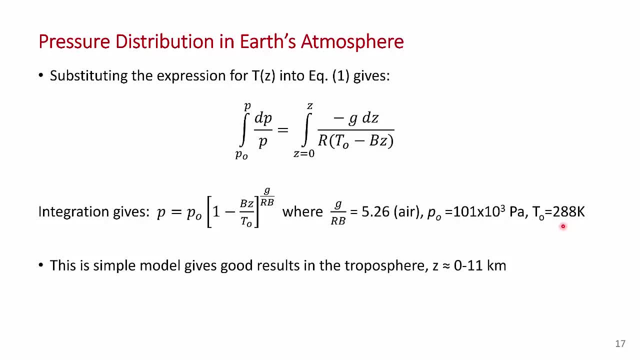 we take the average surface temperature of 15 degrees C, which is 288 k, And that's a really good model of the pressure distribution in the atmosphere as a constant, And then you just divide it by the pressure pressure of the atmosphere And then you just multiply it by the temperature of the atmosphere. 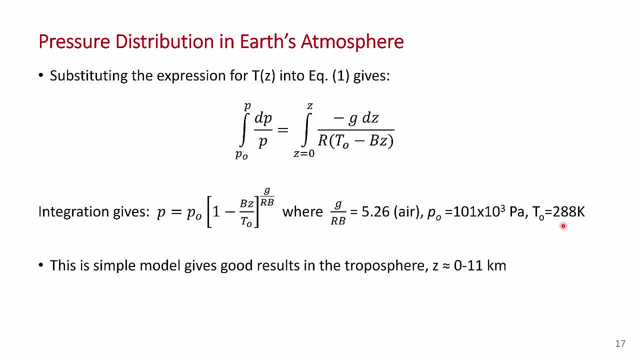 And then you just multiply it by the temperature of the atmosphere, And then you just multiply it by the in the atmosphere, in the troposphere. so in the first 0 to 11 kilometers The key takeaway here- and you know, rather than the detailed mathematics- is that for compressible fluids, if you're going, 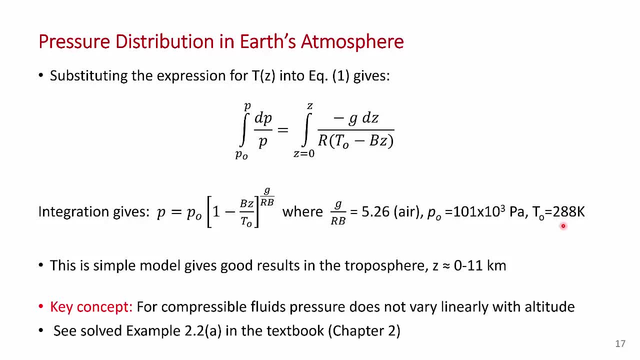 over a large distance because the density varies with temperature and pressure. the pressure distribution is no longer linear with altitude. So have a look. as another example, have a look at example 2.a in your textbook, which uses this equation to actually calculate the pressure at 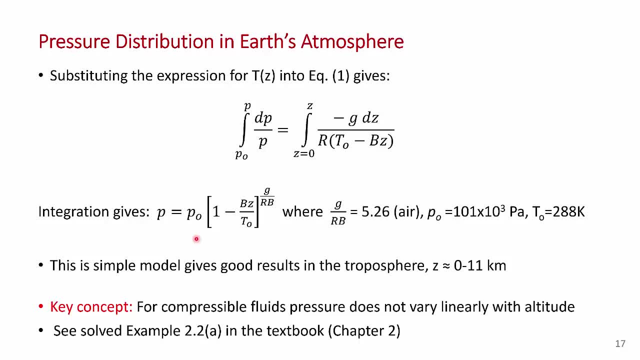 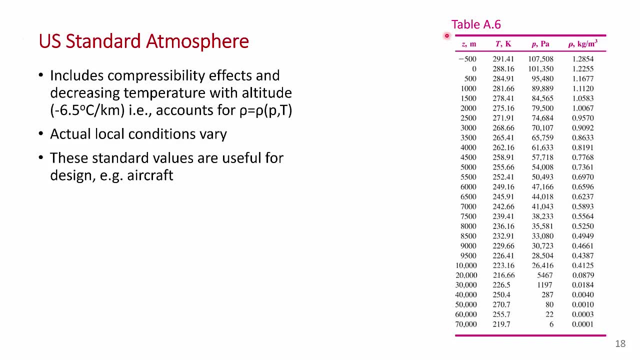 high altitude And this leads nicely to the discussion of the US standard atmosphere Over here. I've shown table 6.. This is from the appendix in your book and it shows the pressure and density of air in the atmosphere going from just slightly below sea level to up to 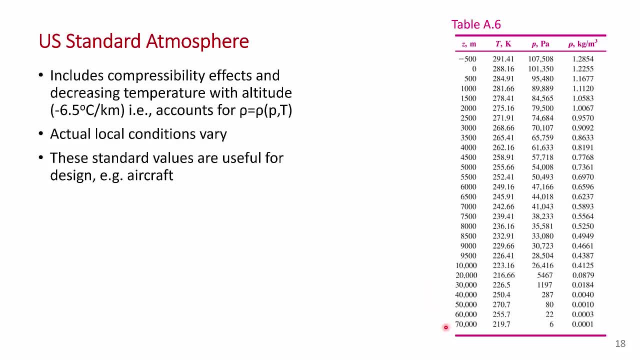 70,000 meters And of course it varies locally with the local weather, but this is a good average approximation of the Earth's atmosphere And it takes into account the fact that air is compressible and that the density of air decreases as you go up in altitude because the pressure decreases. 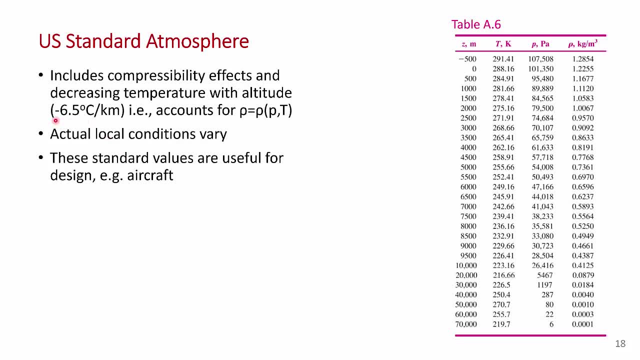 and because of the change of temperature in the atmosphere, the density also changes. So it takes into account the fact that density is a function of the local pressure and temperature. Now, as I mentioned, it varies locally, but these are really good values to use. 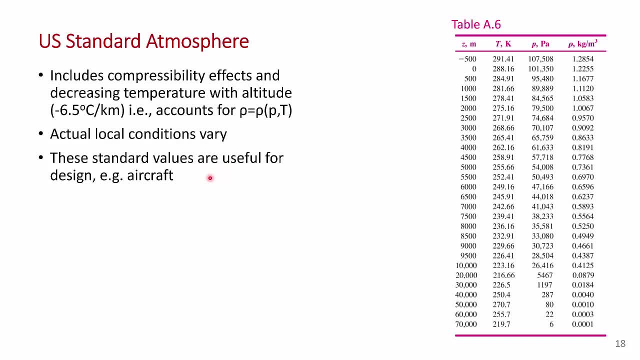 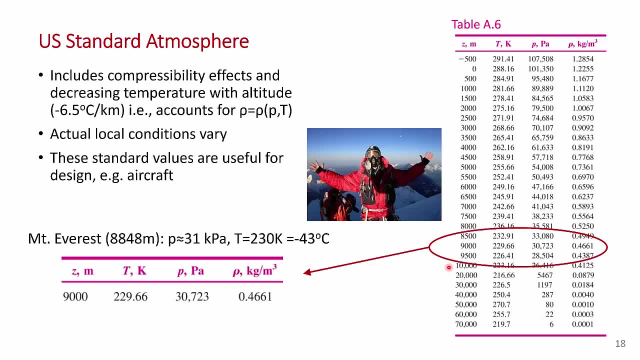 for design purposes, such as in the aerospace industry. If you're looking for a density of air at the cruising altitude of a jetliner, for example, this would be a good place to go And, just out of interest, I've taken the altitude here of 9,000 meters and expanded it. 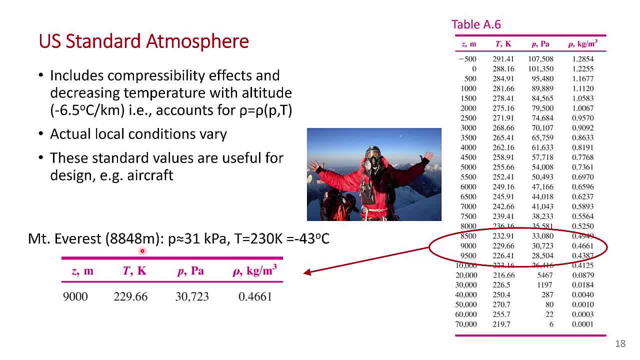 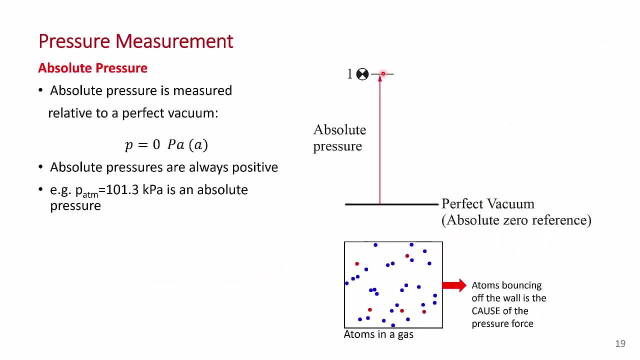 That's approximately the elevation of the peak of Mount Everest, And at the peak of Mount Everest you can see that the pressure is about one third of an atmosphere and the temperature is nice chilly: minus 43 degrees Celsius on average. So next we're going to talk about the measurement of pressure, which is an important topic. 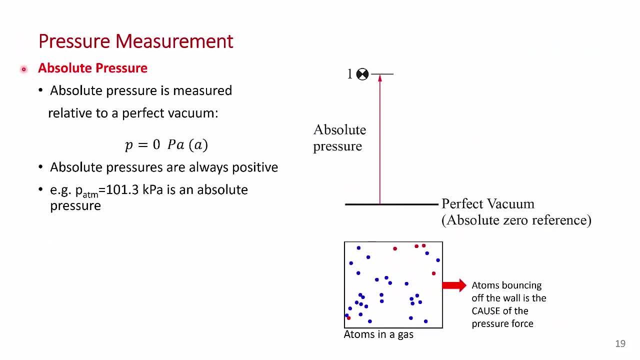 for engineers. But before I can talk about the measurement of pressure, we need to talk about absolute pressure and gauge pressure. Absolute pressure is the pressure measured relative to a perfect vacuum. Now remember that the source of pressure is actually the atoms bouncing against the wall here. So the atoms bouncing against the wall. 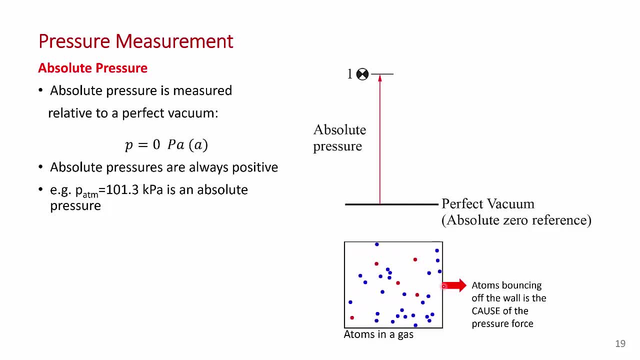 the change in momentum produces a pressure force, And so a perfect vacuum corresponds to getting rid of all of these atoms. So, you know, no substance inside the box, which is a, you know, theoretically not possible, but we can get very close to it. 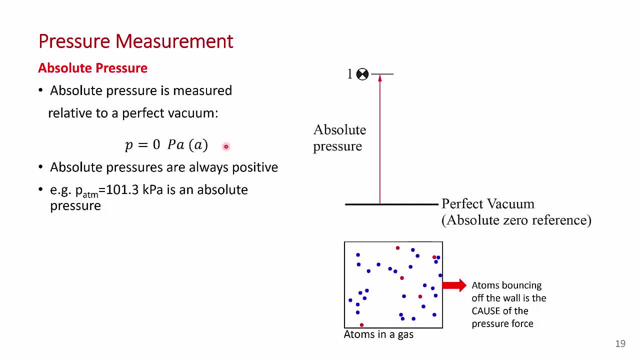 perfect vacuum. So an absolute vacuum. perfect vacuum corresponds to p equals zero pascals, And so absolute pressures are always positive. For example, when you hear that the atmospheric pressure is 101.3 kPa, that's an absolute pressure, So it's measured here, as I'm showing relative to. 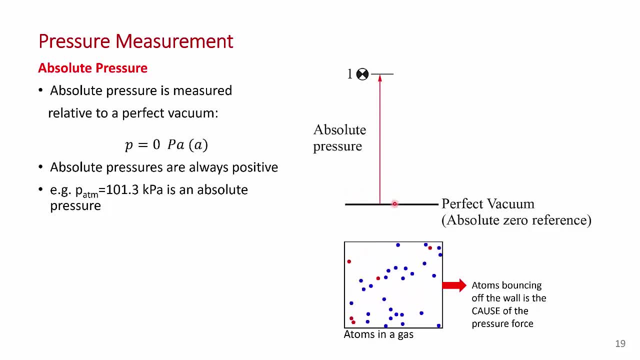 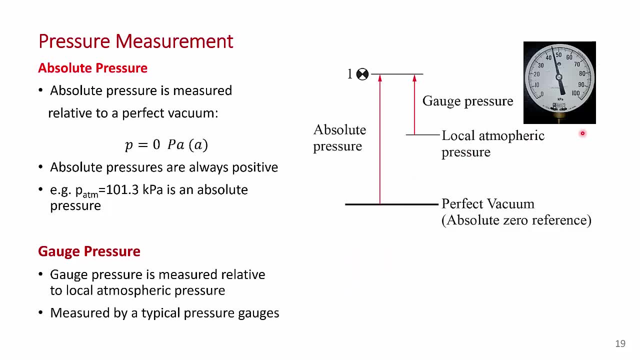 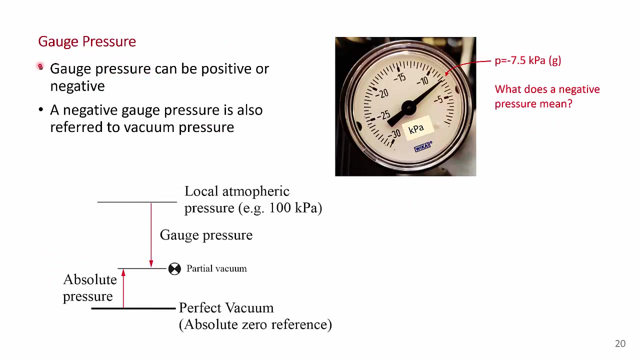 a perfect vacuum. In contrast, there's another type of pressure, called gauge pressure. This is what's measured by a typical pressure gauge that you would see on a tank, And gauge pressure is a measurement of pressure relative to local atmospheric pressure. So, in contrast to absolute pressure, gauge pressures can be positive or negative, And here 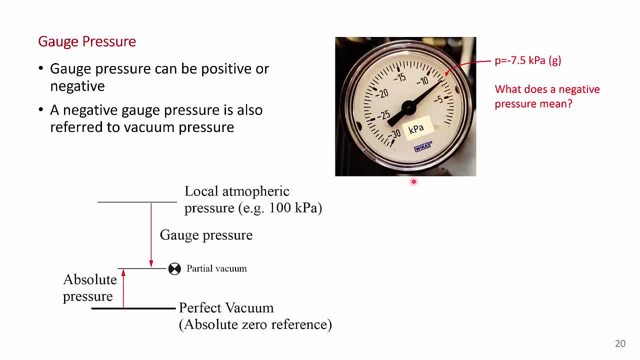 I've shown a pressure gauge. This is actually a pressure gauge off of my camera system, from my underwater camera system, And it's showing- I'm showing here a pressure of about minus 7.5 kPa And I've got the little symbol G here to 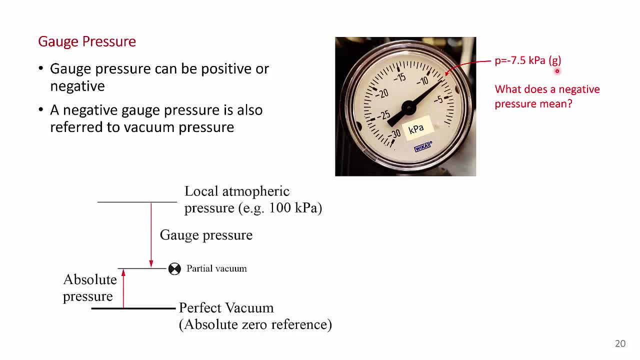 indicate gauge. So what does a negative pressure mean in this context? Well, what it means is that you're below atmospheric pressure. A gauge pressure of zero is atmospheric pressure And a negative gauge pressure refers to a partial vacuum. So again, if we have a perfect vacuum down here, 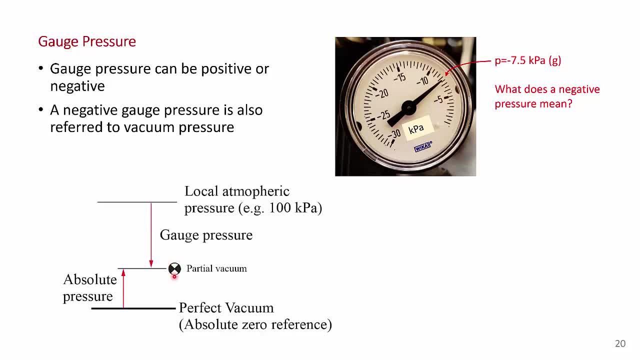 local atmospheric pressure down here, then if we have a pressure that's below atmospheric, a gauge will read negative. Negative gauge pressure is also referred to as a vacuum pressure or a suction pressure. So this is a really important concept and a common source of error that I see in students. 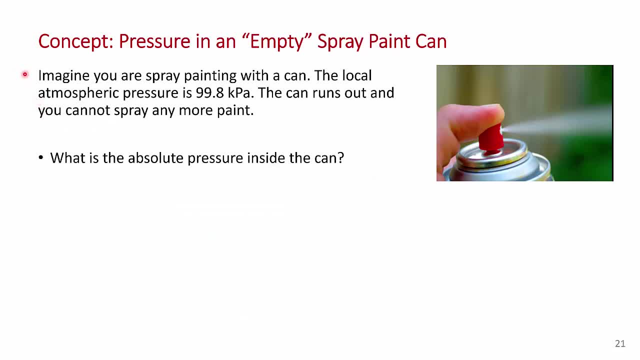 So I just want to talk about this a bit more. So imagine you've bought a can of spray paint and you're spraying it, So I need to put a bit of water and see if it's water, wateragenic, Critical, ERIC. and imagine You've bought a can of spray paint and you're spraying water and story for two and a half feet. 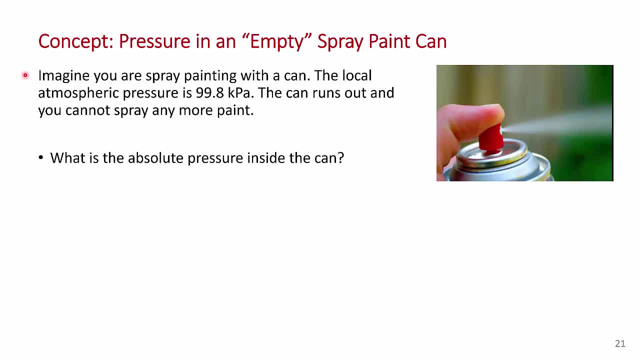 I'm actually trying to track our sleep table right now, so I need to pitcher you out and if you could get a clue to this deifty cath gehen and you're spraying something in your garage and the local atmospheric pressure that day. 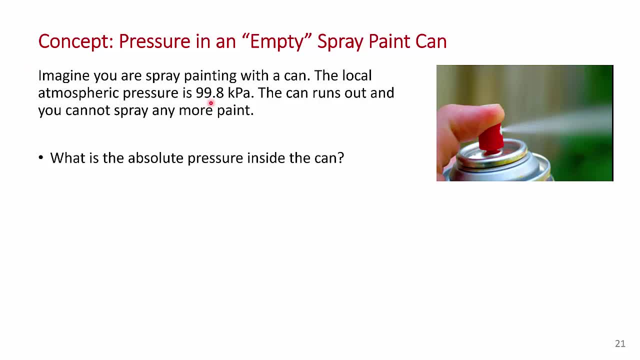 it varies from day to day substantially. So let's say it's a fairly sunny day and the pressure's 99.8 kilopascals and you're spraying the can and it runs out of paint and it can't spray any more paint. 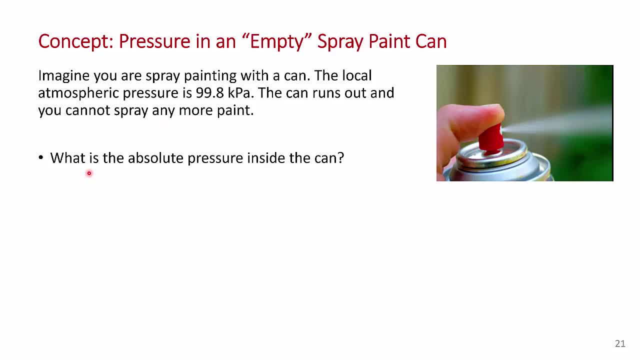 At that moment, you've got the valve pressed down. there's no more paint coming out. What is the absolute pressure inside the can? Think about this for a moment. So what will have happened is because the valve is open, you've got the valve pressed down. 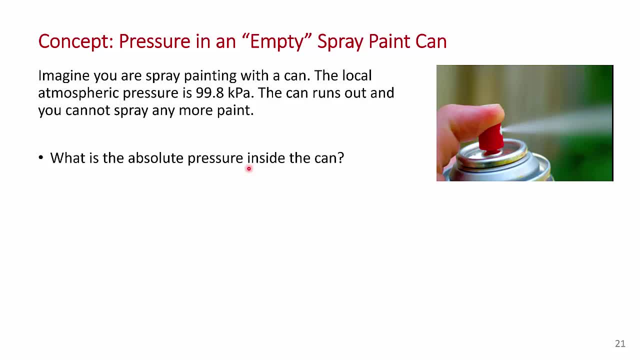 you're going to have equilibrium. The pressure inside the can is going to equal the pressure outside the can. So the absolute pressure inside the can is going to equal atmospheric pressure, So 99.8 kPa, and we often use this little symbol A. 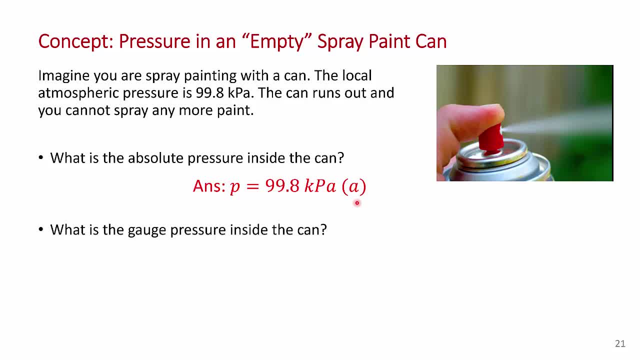 to represent absolute pressure. So what is the gauge pressure inside the can? If you were to attach a gauge to this, to this can, what would it read? Think about that for a moment. So the answer is that the gauge pressure, because gauge pressure is relative. 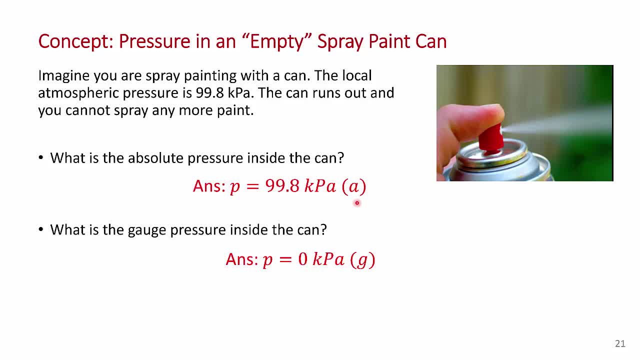 to local atmospheric pressure. the gauge pressure is zero. We use this little symbol here to indicate gauge. So if you were to attach a standard Borden gauge- and I'll talk about how those work in a minute- to the outside of this can. 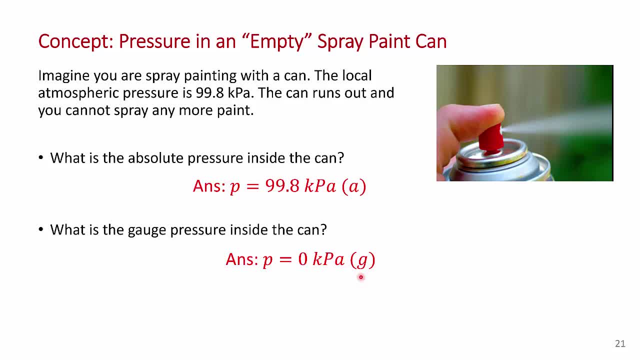 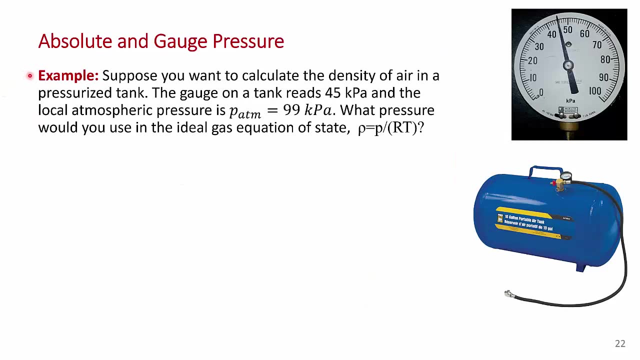 you know, through the wall of the can it would read zero. An empty can still contains propellant at local atmospheric pressure. So let's come to a specific example here, And this is an example that I- where I see student errors a lot. 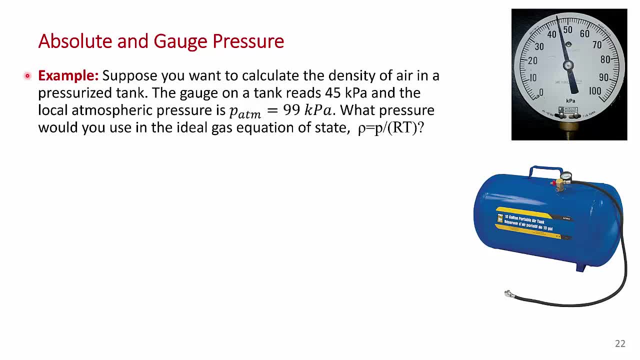 And it's a place where you could make a big error if you didn't understand the difference between absolute and gauge pressure. So the question states: suppose you want to calculate the density of air and the temperature of the air In a pressurized tank? 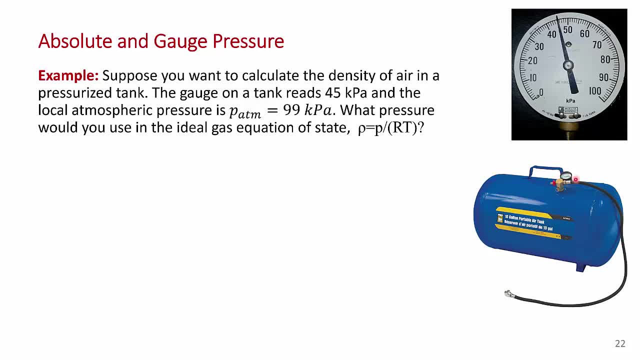 the gauge, and I've shown a tank over here with a gauge on it. So the gauge on this tank reads 45 kPa and the local atmospheric pressure is 99 kPa. We covered this in chapter one, right? So we want to calculate density here as P over RT. 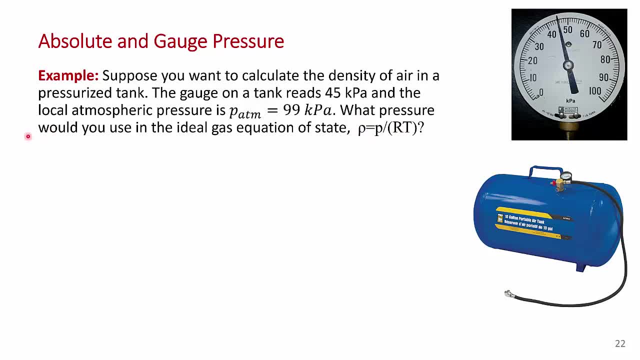 The question that I have is: what pressure would you use in the ideal gas equation of state? Think about this for a minute. You might want to pause the video. The answer is: you want to use the absolute pressure. You must use the absolute pressure. 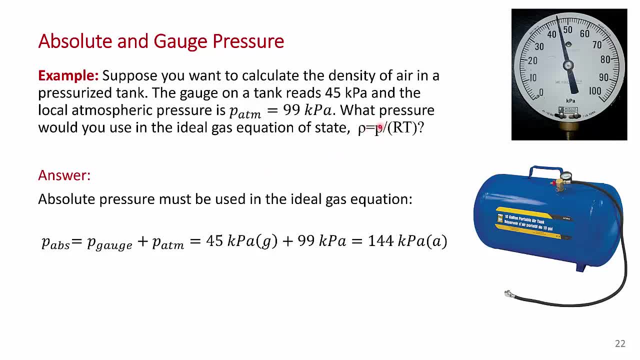 in the ideal gas equation of state. So the absolute pressure is the gauge pressure plus the atmospheric pressure. So you take the 45 kPa and add on 99 kPa and you get 144 kilopascals. So that's the number that would go into. 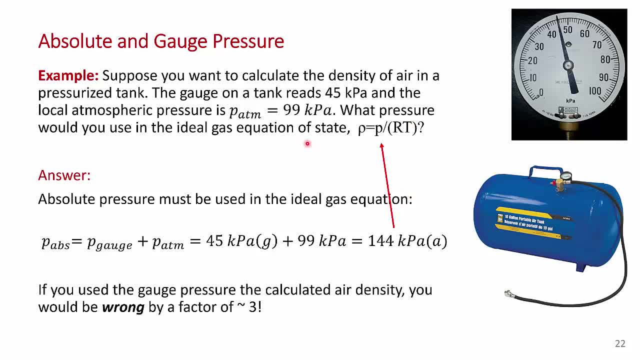 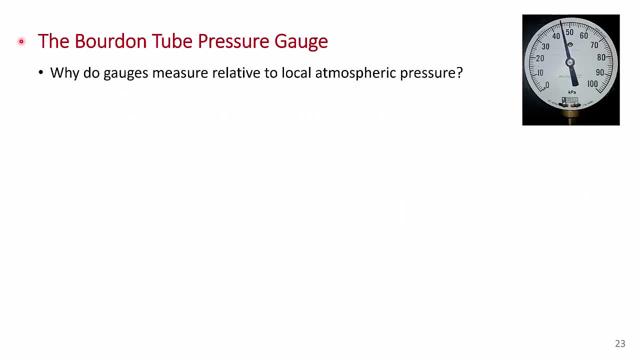 the ideal gas equation of state. If you just read the gauge 45 kPa and put that into this equation, you would get an air density that's out by more than a factor of three. Okay, so you might wonder why these gauges? 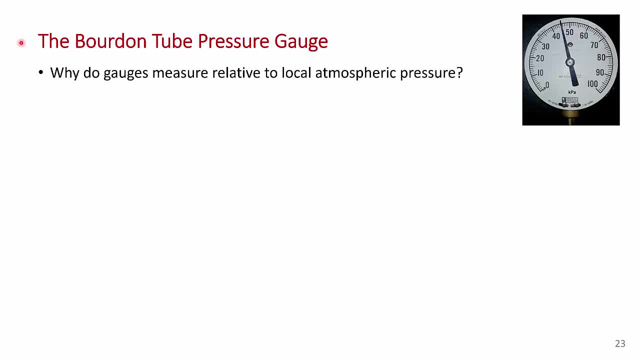 why do they measure relative to local atmospheric pressure? I really want to address that, because I think it's one of those things where it's so easy to make an error if you don't understand, So the reason these Borden gauges measure relative to atmospheric pressure. 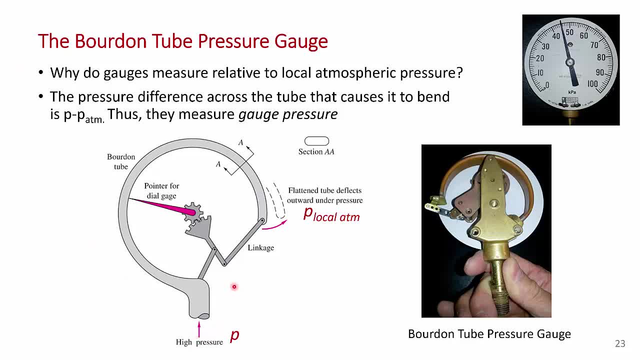 is because of, well, their design. They're just a bent piece of tubing and this is a hollow tube. that's showing the cross-section here, and this bottom of the tube here is connected to the pressure that you want to measure, and when you pressurize this tube, it wants to straighten out. 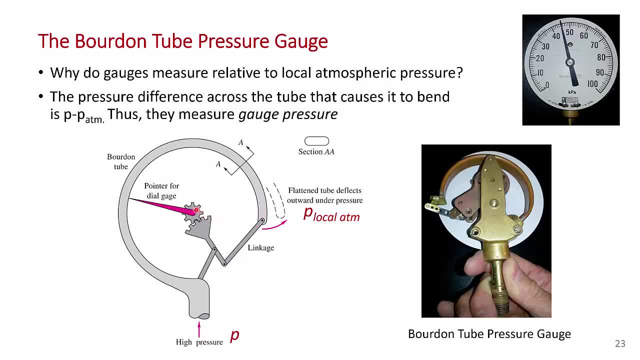 and and that deflection here is attached to a linkage that indicates the pressure, And so it's the difference between the pressure inside the tube and local atmospheric pressure that produces the deflection that makes the dial move. So if this pressure here was atmospheric pressure, 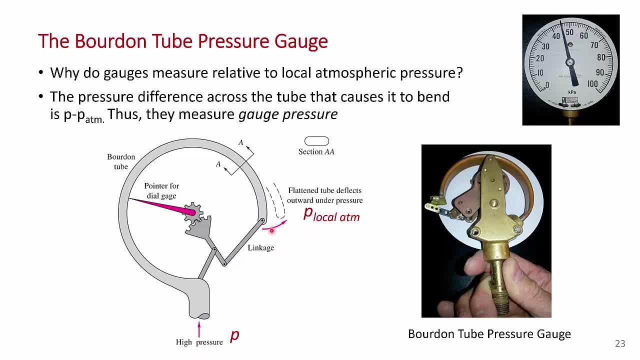 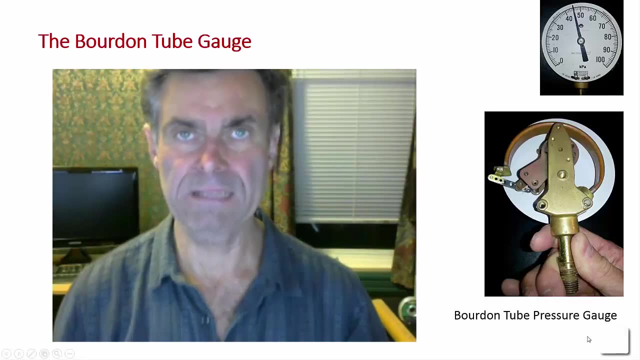 that would be the same pressure as the outside of the tube and you would get no deflection and the gauge would read zero. So hopefully that explains why Borden gauges measure relative to local atmospheric pressure. Okay, let's give this a shot. 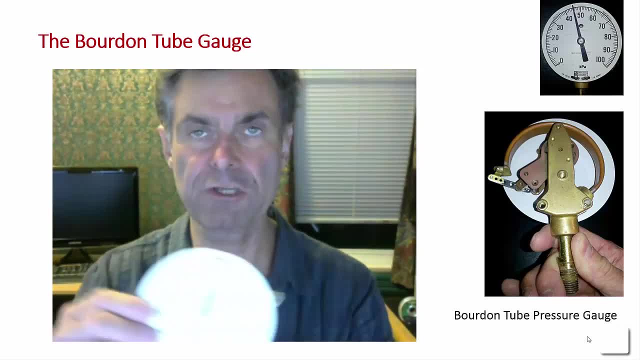 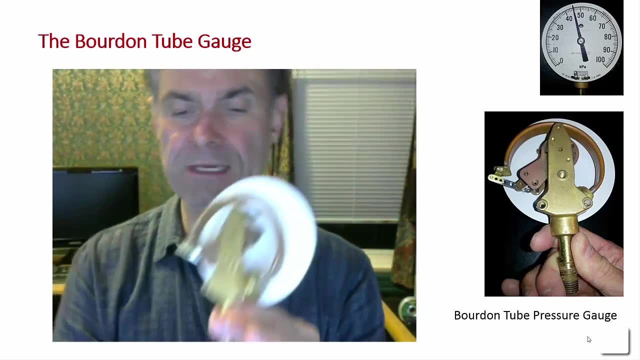 In case the previous slide wasn't clear enough, I just wanted to show you a stripped-down Borden gauge And hopefully you can see this. Here's the flat hollow tube that gets pressurized from the attachment, And what happens when it's pressurized is it wants to straighten out? 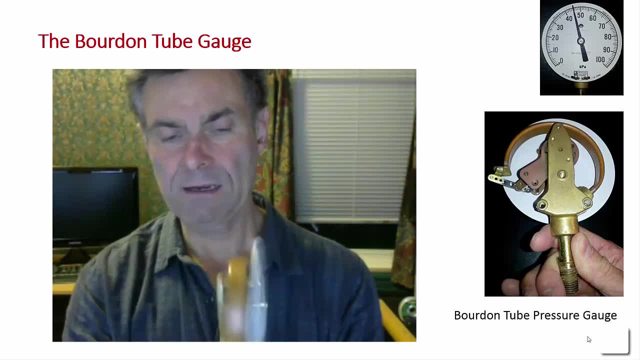 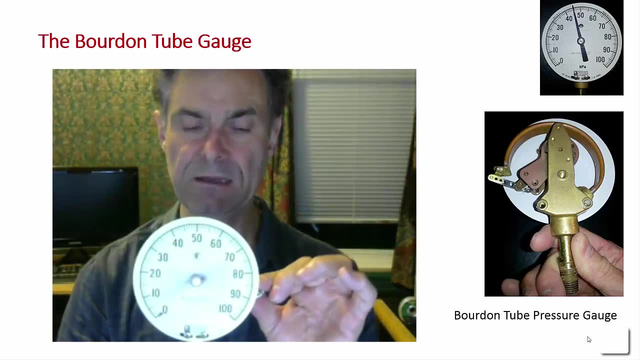 So this end flexes And I'm going to turn it around and you can see when I flex it. I'm going to simulate. I'm going to simulate the internal pressure by flexing it with my finger and you can see that the needle move. 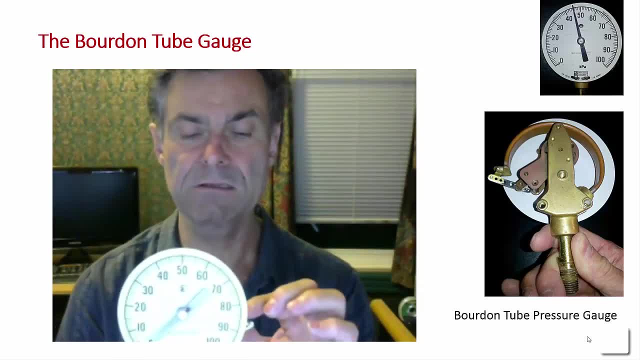 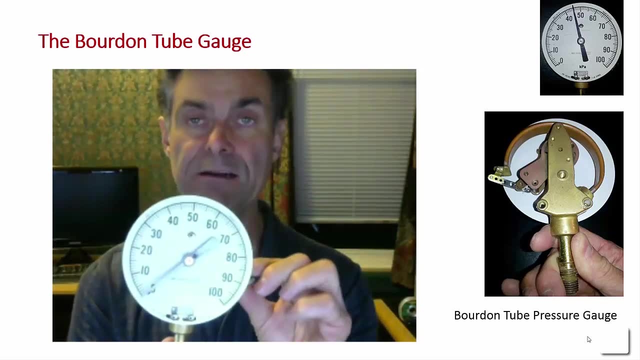 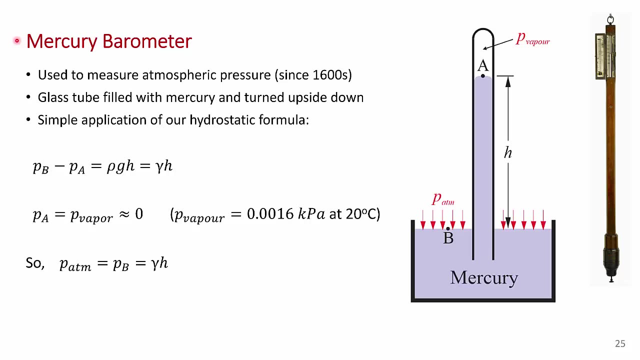 And provided you're in the linear elastic range, the deflection is going to be linearly proportional to the internal pressure. So hopefully that clarifies how a Borden gauge works. Okay, next I'd like to talk about mercury barometers. Mercury barometers measure absolute pressure. 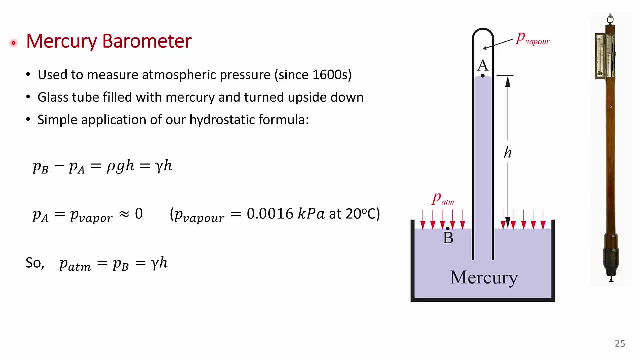 You've probably used one of these in the labs. If you did a chemistry lab, you may have measured the pressure with a standard mercury barometer that I've shown over here. So they've been used to measure atmospheric pressure since they were invented in the mid-1600s. 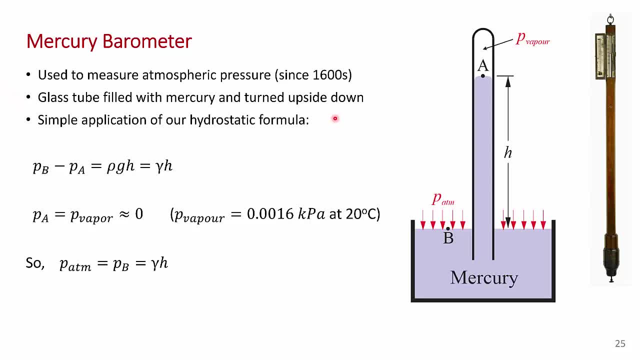 And what they are is a glass tube filled with mercury, and then they're turned upside down and you get this void here Now. it has a little bit of mercury in there, because mercury does have a vapor pressure at room temperature, but that's incredibly small. 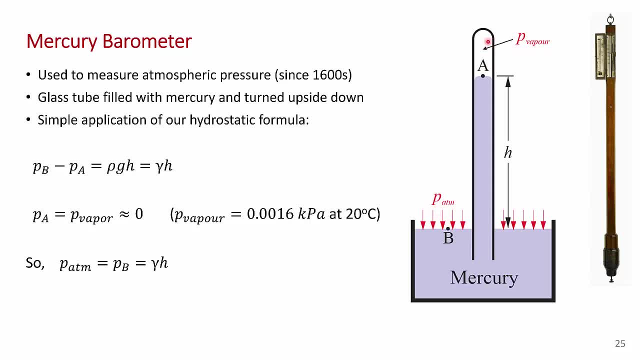 And so atmospheric pressure acts on the surface here, and the pressure here is very, very low. And so we can, using our hydrostatic equation for an incompressible fluid, we can say that the pressure difference Pb minus Pa, Pb is atmospheric pressure minus Pa. 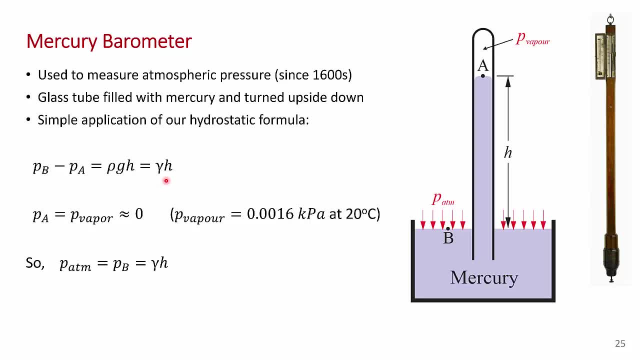 is equal to gamma of the mercury times H, And I just mentioned that the pressure at A, here the vapor pressure of mercury is very low. It's equal to 0.0016 kilopascals Kilopascals at 20 degrees C. 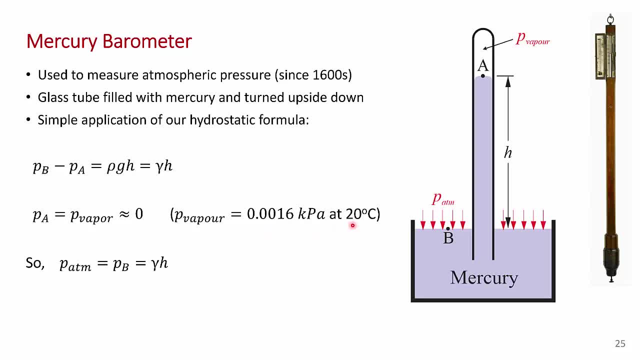 So it's close to a perfect vacuum- Not quite, of course, but we can approximate this as zero. So we can just say that the atmospheric pressure is equal to the pressure of B equals gamma H, And so that's a nice way to measure atmospheric pressure.